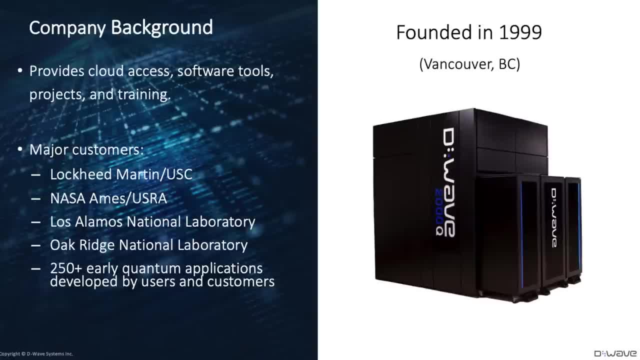 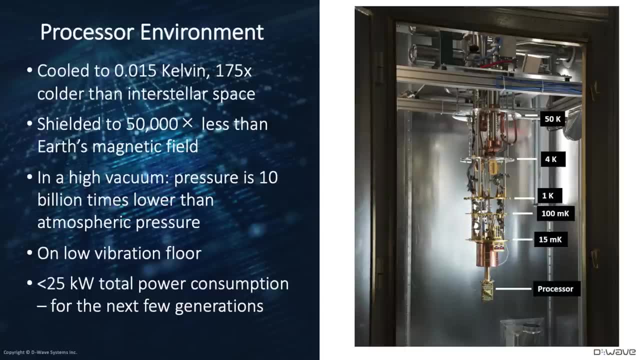 and I'm hoping that I can get you interested to write some of those as we go forward into the future. And now let's talk a little bit about what happens when you open the door of one of those D-Wave quantum computers that you saw. 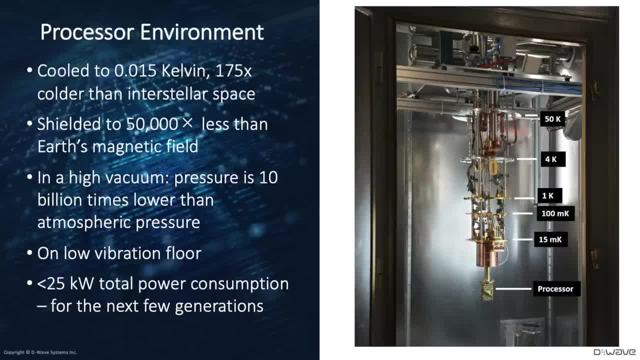 You have to keep a very careful environment inside for the QPU, the Quantum Processing Unit. The environment has to be cooled as close to absolute zero as you can get, In our case 10, 15 millikelvin, so that the effects of heat do not play a role in the operation of the chip. 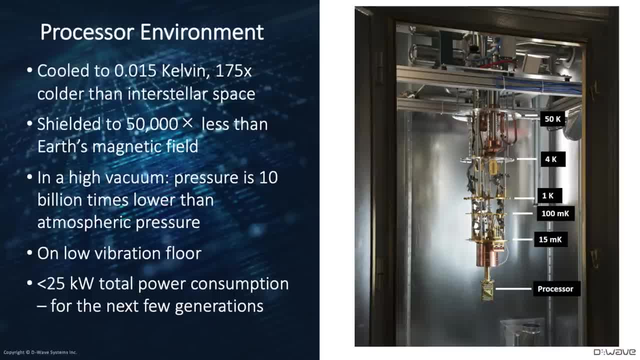 In other words, you want the chip to operate as quantum as possible, which means you have to shield out the effects of heat. You also have to remove as much heat as possible, remove as much of the radio frequency interference, magnetic electric fields and so on. 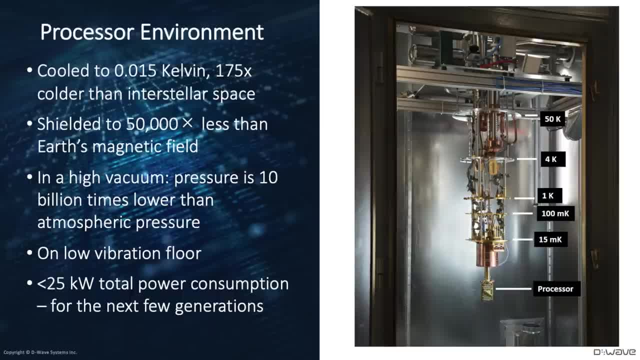 as much as you can, And you also have to pump everything out to try to get it into a vacuum. So the pressure has to be way lower than atmospheric pressure in order to be able to get the quantum effects to occur without collisions with particles in there. that would interfere with the quantum effects. 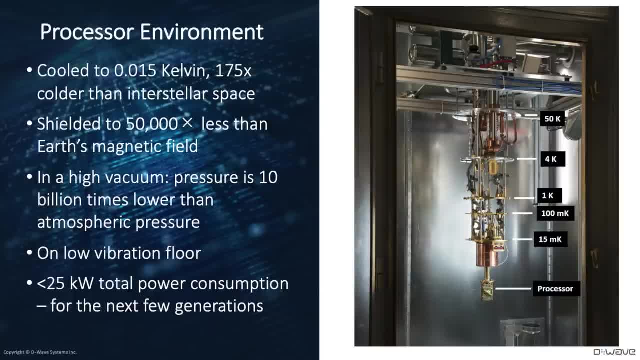 It is put on a low vibration fan and you have to do it carefully. Basically, when we install, we go through a process of hardening or putting in a new floor, And one important point about the D-Wave QPU is that the total power consumption is very low. 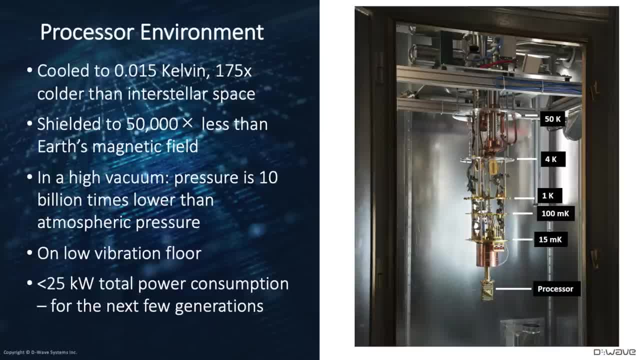 by the comparison to HPC machines, which take up entire rooms and need their own power centers. These machines, these quantum computers, need very little power. Your main power is really for the refrigerator, And so it's going to be interesting, in my opinion. 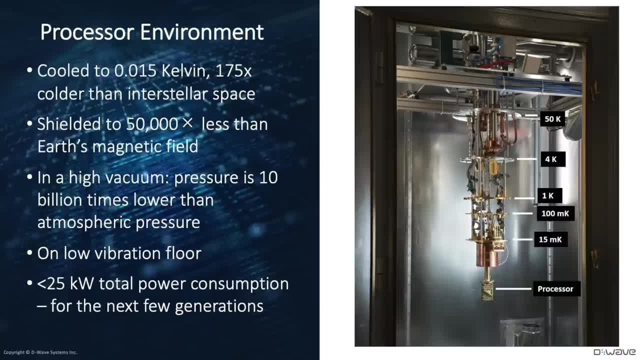 to see how this competes, as these HPC systems keep getting bigger and bigger. That's not going to scale going forward in a world where there's not enough power, So I think quantum will offer a good option for that. Now I want to focus your attention to the right here. 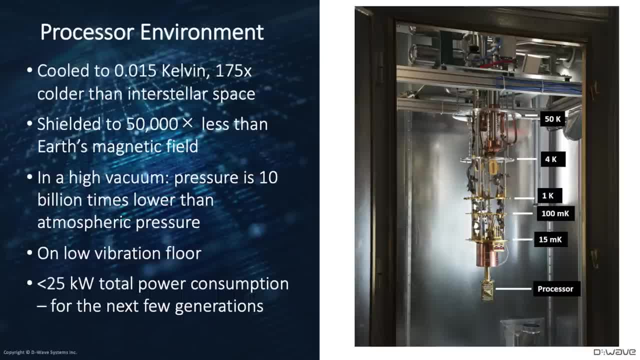 that inverted finger, if you will, is the chip. The QPU itself is placed at the very bottom and you have several levels of temperature. that the refrigerator works in a staged process, meaning that at the top it can be room temperature and then, as you go, you have liquid nitrogen and liquid helium. 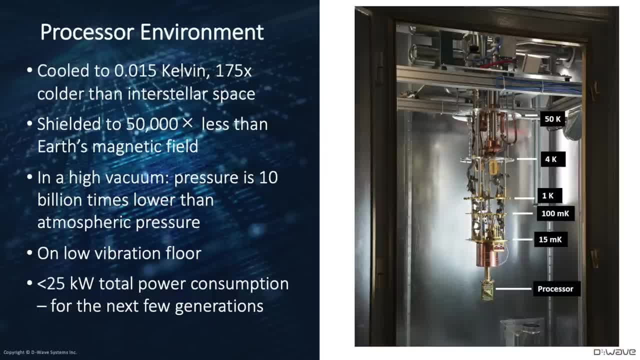 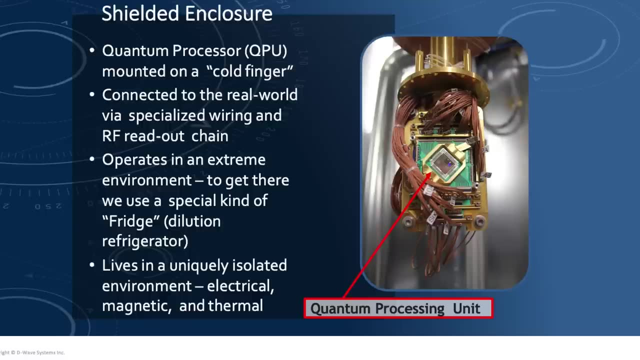 on down Until finally, at the bottom, you have your millikelvin temperature layer and there's of course, a lot of wiring to get the signals in and out, And this slide kind of brings it together a little more to show you the environment that it's in. 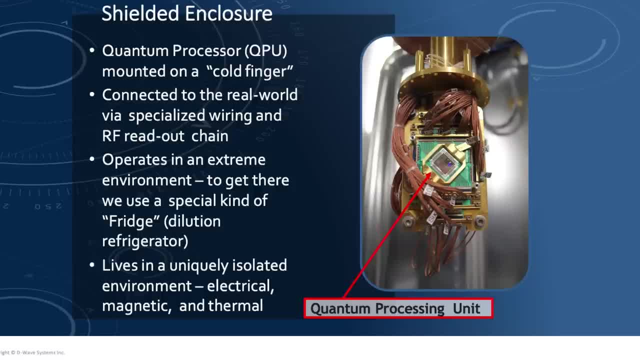 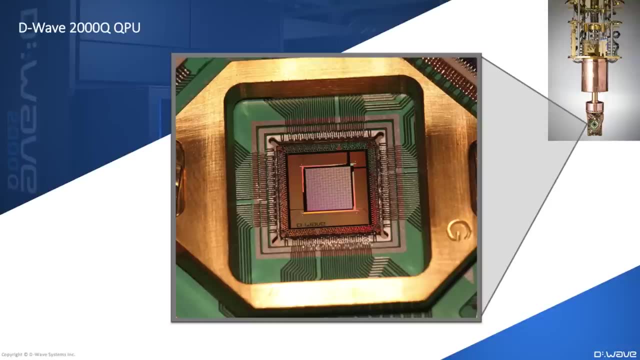 with all the wiring and so forth at the bottom. But basically you have to keep the chip in a very, very uniquely isolated environment with a lot of requirements In order for it to behave as quantum as possible. And here's a close-up of the D-Wave 2000Q chip. 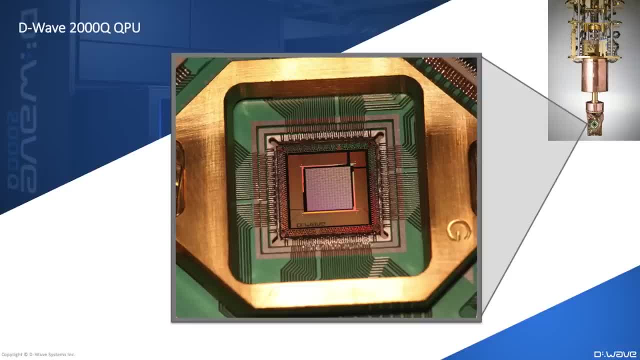 It's to get a sense of the scale. It's on the size, on the order- excuse me of your fingernail, of the thumb- And so you can see the wiring on all four sides and so forth, And hopefully now you've gotten a feel for what's inside the box. 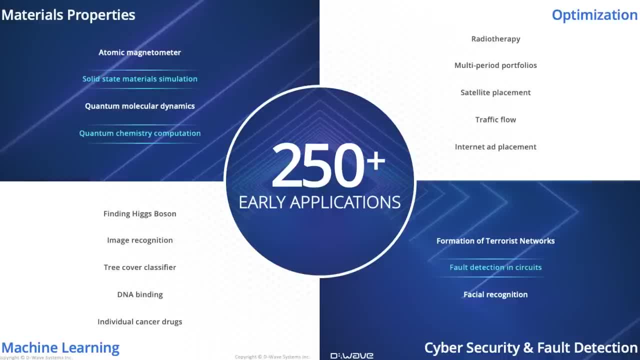 And, as I mentioned earlier, we've seen at least 250 early applications of quantum problems which have been solved and explored on the quantum computer and also our hybrid solvers, which we'll be talking about in the additional materials and the other tutorials. But I just want to mention a few of these. 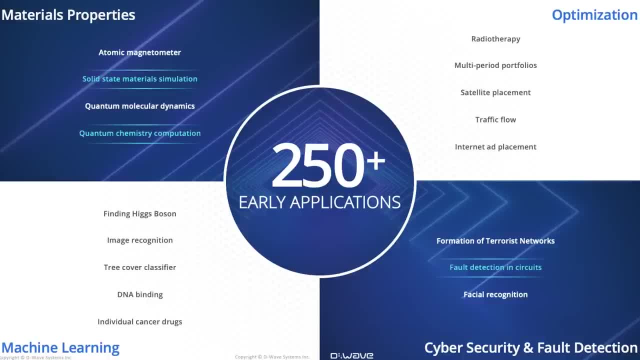 because to me they're really interesting. They're very diverse Topics like formation of terrorist networks, facial recognition, radiotherapy, traffic flow, finding the Higgs boson as a high-energy physics example, And recently people have been studying how they can use the quantum computer. 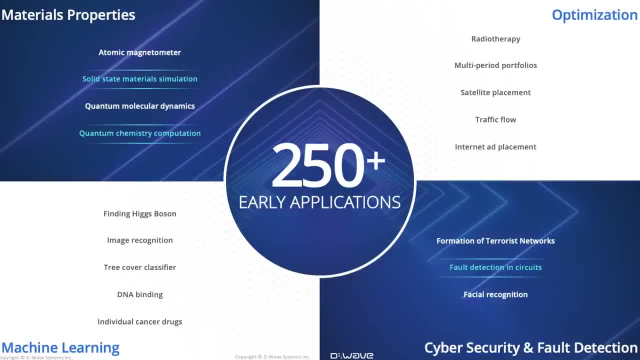 to help with the search for solutions to the overall problem of COVID-19.. And these applications are getting to where they're becoming production size- which is even more interesting, because that's been one of the criticisms of quantum for a long time- is that, oh, it's too small, and so on. 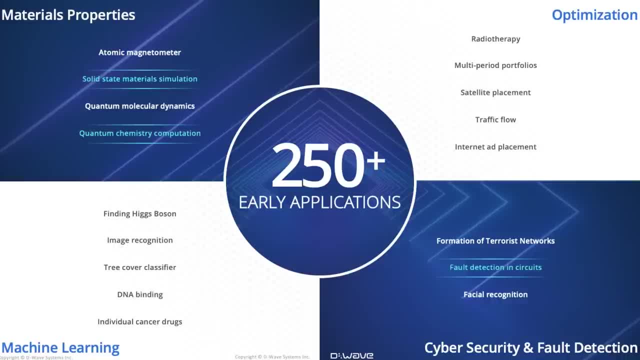 You can't really solve any problems yet, And I'd like to show you in this tutorial that that's not the case. I wanted to mention also one cool thing that Los Alamos National Laboratory did, which was that when they first got their machine, 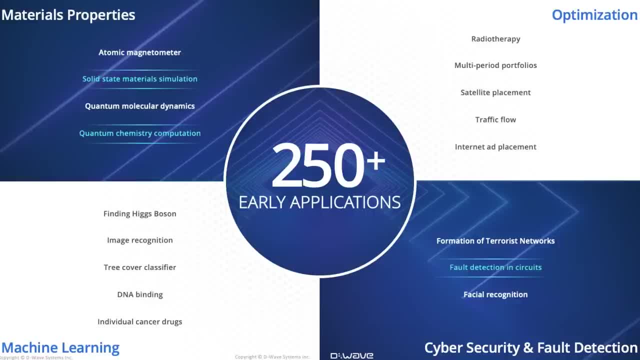 they made it available to their researchers with just a few paragraphs about what they wanted to do would get them some time, And that produced a tremendous number of things. But one of the things I also enjoy about my own current job is that papers appear almost every day. 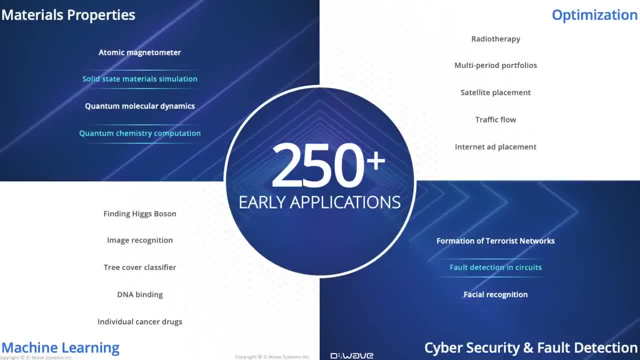 where someone has done something interesting with a D-Wave quantum computer or, for that matter, one of our competitors' quantum computers, And I just find that fascinating. I think we're all waiting for the killer app, But in the meantime I want to convey to you: 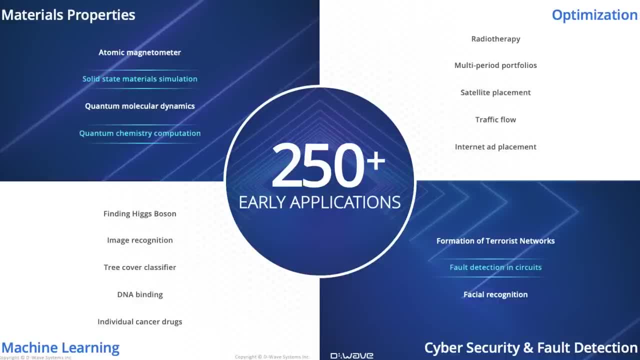 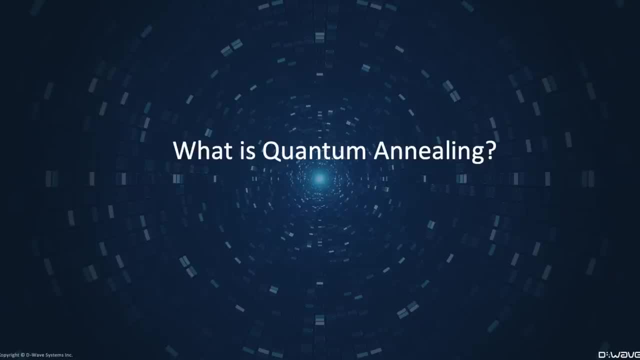 that quite a lot of work is going on at the moment. So let's move on now and start digging into the D-Wave environment and quantum computer, And the first thing to mention is the subject of quantum annealing. Now, you might be familiar with the fact. 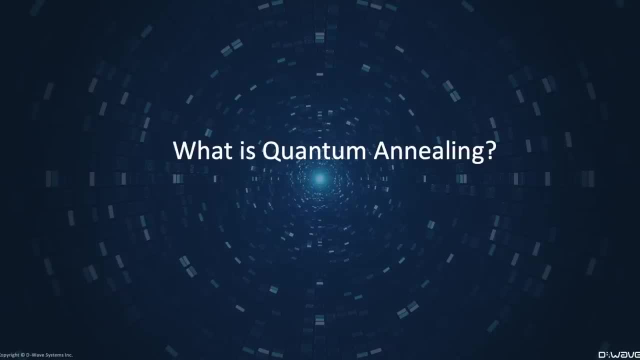 that there are basically two ways to build quantum computers that have been proposed and implemented so far: the gate model and quantum annealing. And D-Wave took the quantum annealing route. So let's discuss that. What is quantum annealing? And the first thing I want to mention: 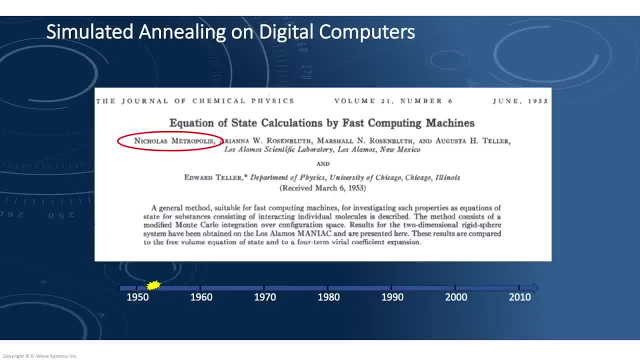 takes us back to a very influential paper from the early 1950s which brings forth work that was done for the atomic and hydrogen bombs at Los Alamos and then later at Livermore, And this particular paper by Nick Metropolis and including Edward Teller. 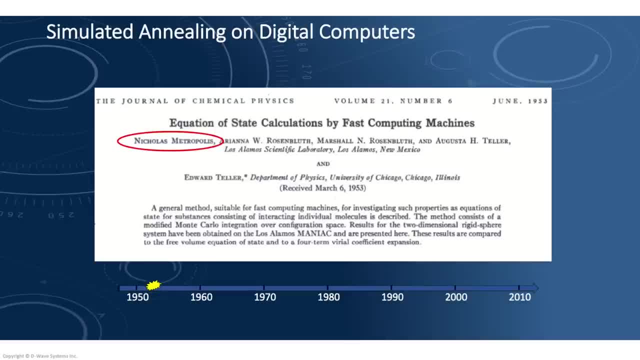 basically puts out the beginnings of these numerical computations. We're going to talk a little bit about simulated annealing and quantum annealing, But it's important first to recognize that this field is still in its infancy, This paper, which was very influential and started all this. 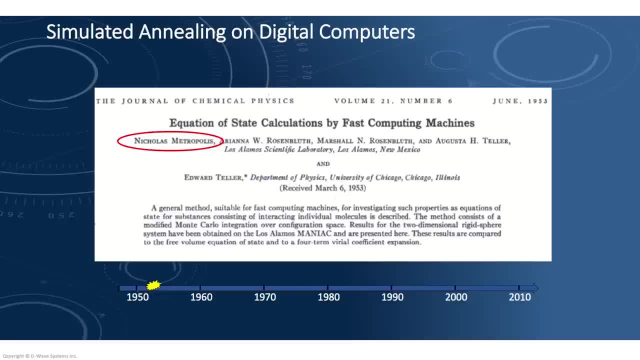 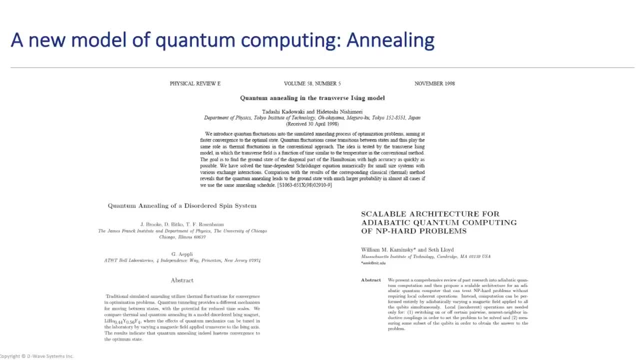 is only from the 50s, which is really not very long ago, And the paper that got everything started was in 1998 from two Japanese physicists, Nishimori-san and his student Katawaki-san, And this paper suggested: 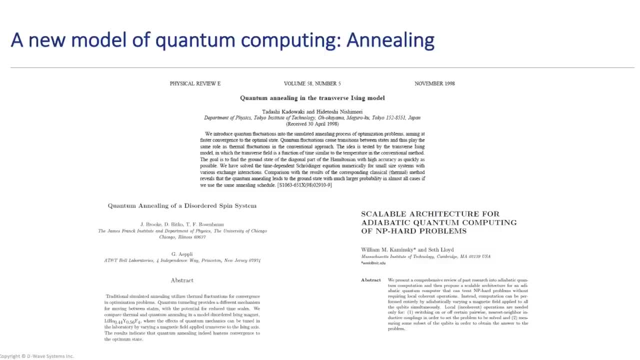 the algorithm of quantum annealing, And you can see here I've included on the slide a couple other influential papers, notably by Seth Lloyd, down there below on the right, And the main contribution of this paper, as I see it, was to suggest: 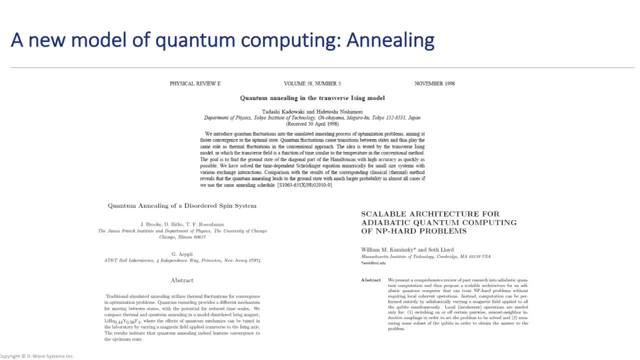 that it might be possible to build a quantum computer which could find the ground state of a system that's built into what's called the transverse Ising model, and we'll get into that in a little while, And I want to mention a few things more. 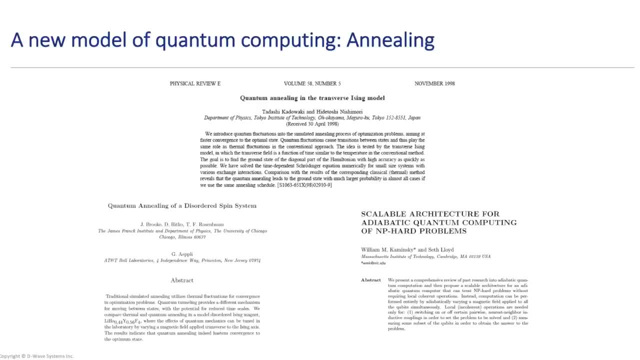 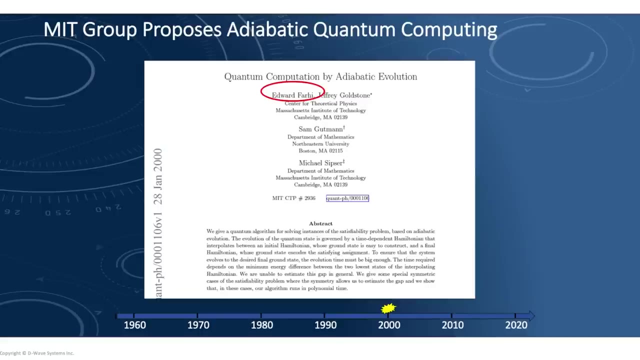 about annealing first, in order to understand that You don't need to really understand very much of this at all in order to operate and use and solve problems on the quantum computer, though. So this is really all background, And what came next after the Katawaki-Nishimori paper. 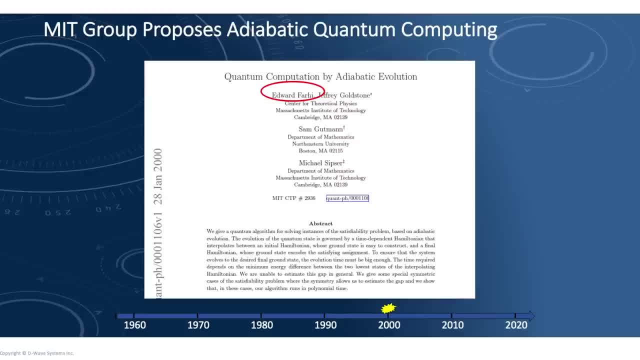 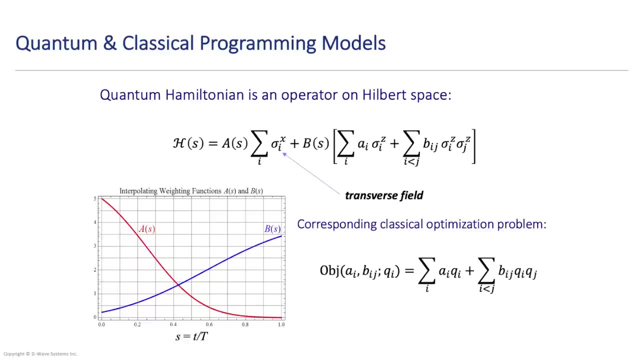 was a contribution by Eddie Farhi a few years later, basically laying out a procedure of what they called adiabatic quantum optimization. And here's one slide where we've basically boiled down a lot of the physics. And again, like I said, 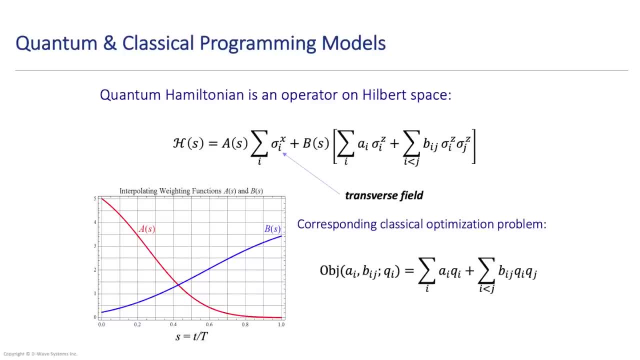 you don't really need to know these things. This is more for background, And if you are a physicist out there and you're interested in the details, there's papers and physical review that we can point you to to give you a lot more of the detail. 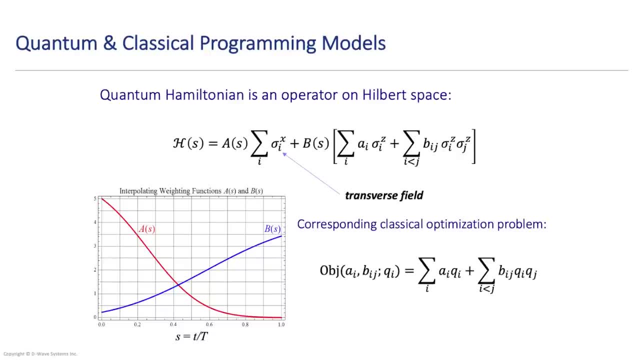 But the idea is you start with this thing called a Hamiltonian operating on Hilbert space, And it basically has two terms: the A of S, which corresponds to an original wave function. it's called where all the qubits are kind of in a cloud. 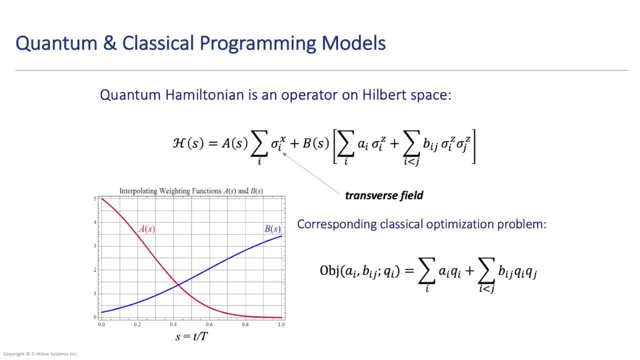 of up and down states And the B term, the B of S, is the problem that the user wants to solve, And the idea behind quantum annealing is that during this annealing cycle it's called you turn down the initial state. 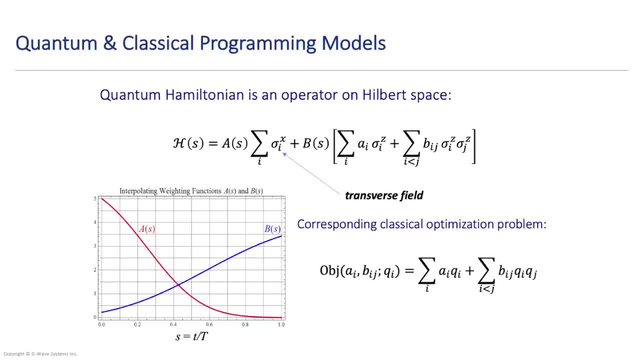 which is controlled by this transverse field, and you turn up the final state so that at the end of the cycle, if you do this slowly enough and under what are called adiabatic conditions, you will find that the system in the ground state. 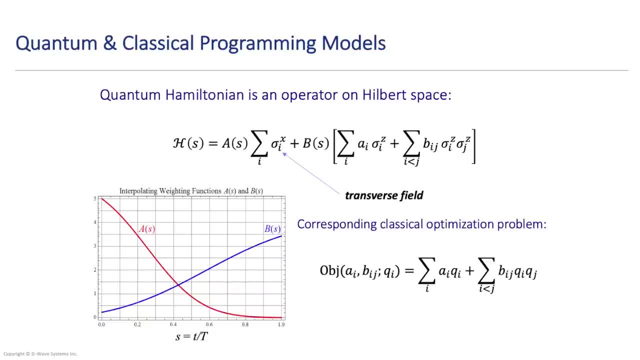 that is the lowest possible energy, And the way it gets manifested in a programming sense is that that Hamiltonian gets basically transformed into, in the lower right, what is called an objective function in a corresponding classical problem which has these numbers called A's and B's. 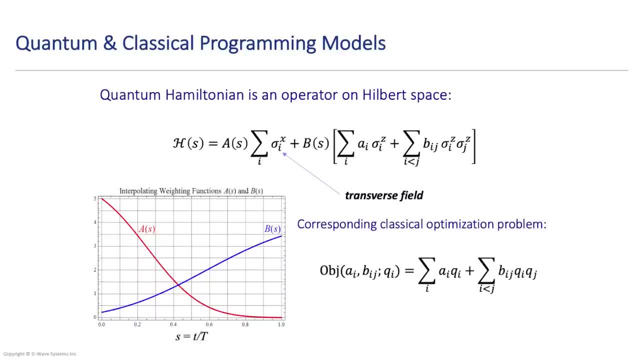 and qubit variables, Q sub I, as you can see there, And we're going to talk now more about those terms. So we're going to leave the physics behind and focus in on the term that it's been, on the problem it's been. 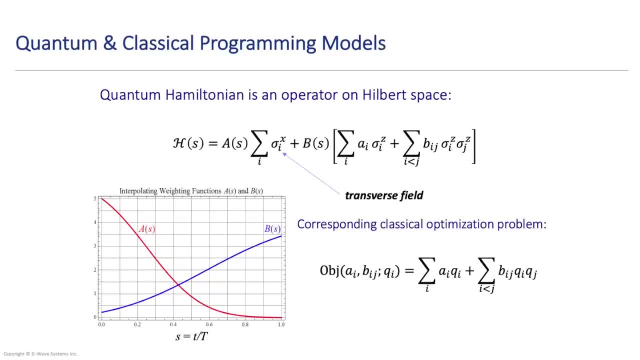 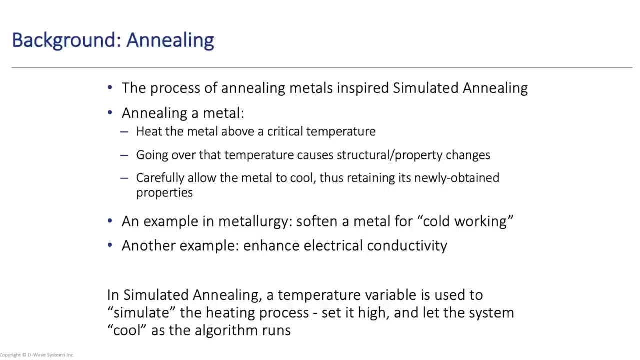 transformed into with the qubit variables And so this process. it turns out that where you turn up the one problem or change the parameters in it and gradually turn down the other, was used in an analogy with the notion of annealing as it had come forward. 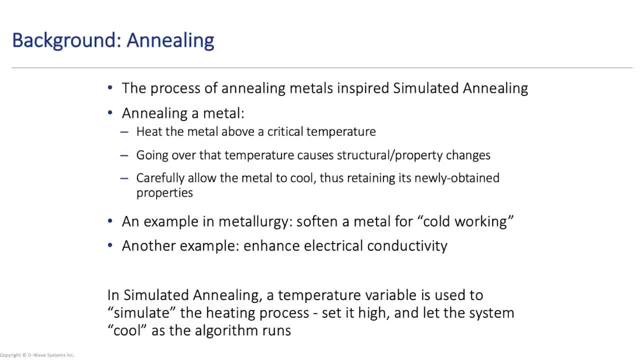 in history And, just briefly, the process of annealing metals is where that came from, And what that means in metals is that you take a piece of metal and heat it over a critical temperature And when you go over that temperature you cause structural property changes. 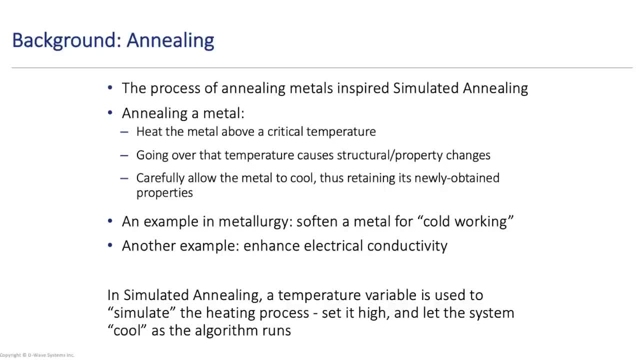 to occur, And then you cool it under certain conditions, And if you do that and you do it carefully, you can end up with properties in the metal that are different than you had before, And so something might be cold worked. it's called. 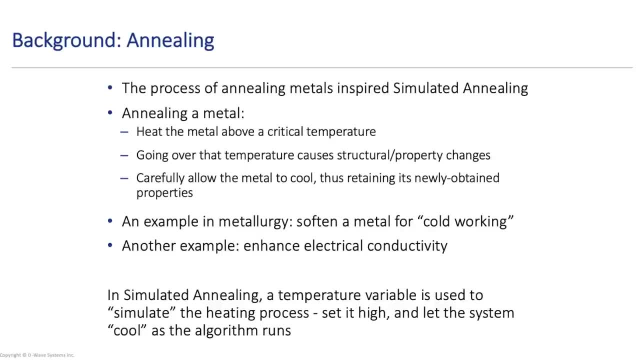 cold working, Or you can enhance the electrical conductivity, And people had developed this a long time ago in making swords and things like that. So this came up then in simulated annealing, which was a numerical algorithm developed decades ago, where you have 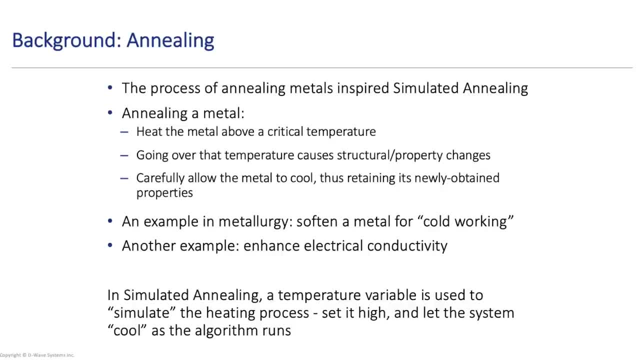 a temperature variable and you simulate a heating process, set it high and let the system cool as the algorithm runs. And so, in our case, this process of starting the system in one state and then gradually turning up the end state and turning down the beginning state, 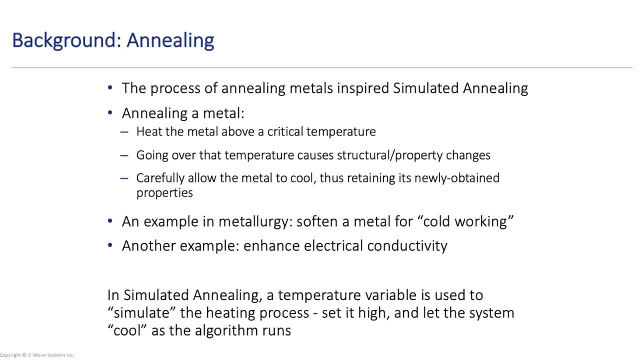 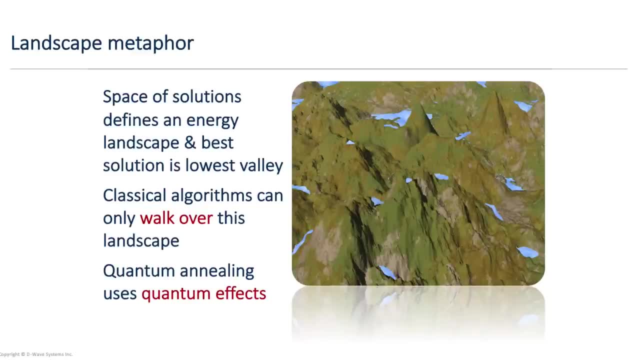 is called quantum annealing, And so that's where the name came from, And so this picture of turning up one turning down the other also has another metaphor that we can use, And this is probably more useful for you to keep this in your head. 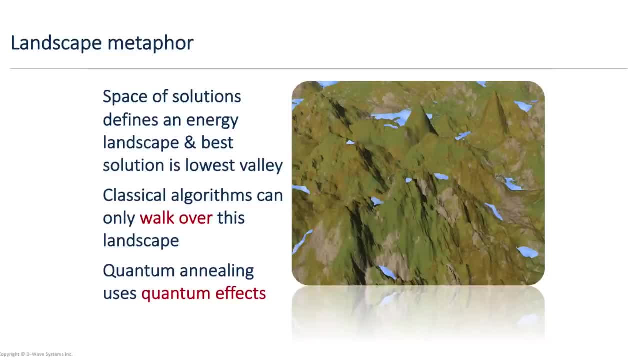 because it's going to be important as we go forward and we start to actually build our own problems and solve them, Which is that the space of solutions. for that end state that I talked about defines an energy landscape, And so you can picture a mountain range. 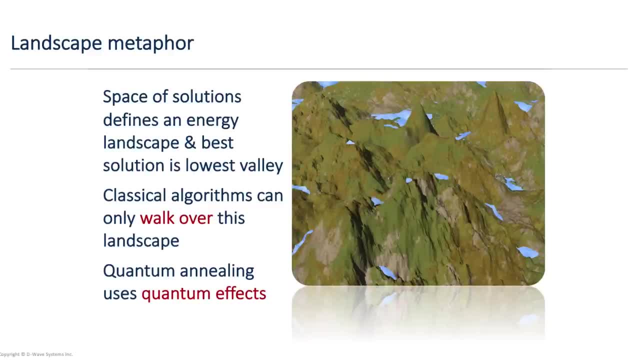 with peaks and valleys, And your basic goal is to try to find the lowest energy state that you can. In other words, where's the valley, Where's the lowest valley, Not just some intermediate valley which might be locally low, but not all the way low? 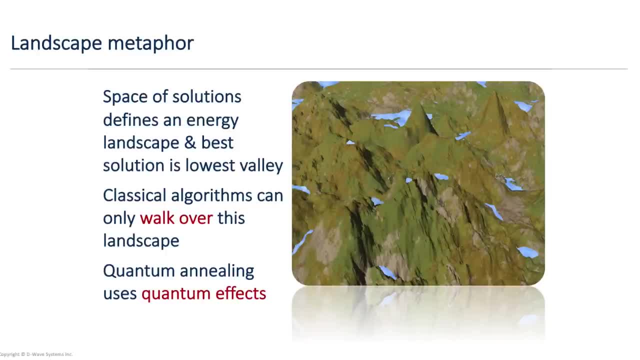 Where is the lowest energy that you can find? And the analogy in the quantum case and what was called quantum annealing is that classical algorithms can only walk through. So if we're hikers out there, we have to walk all the way up to the top of the peak. 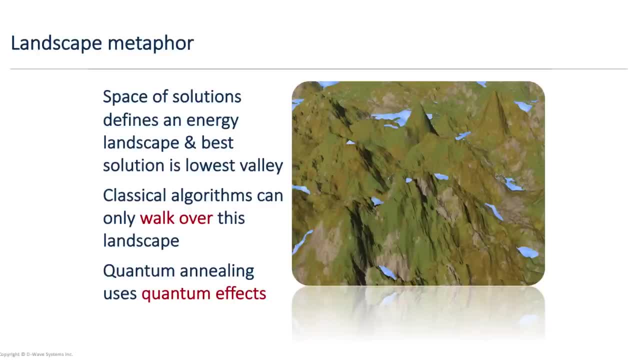 in order to get to the other side, Whereas in quantum physics there's some finite probability of tunneling through the barrier. That's an example of one of the quantum effects on the slide here You have the possibility of doing. that Especially depends on 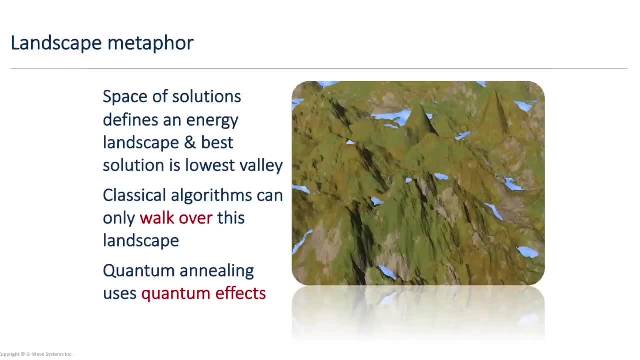 how steep the peak is and how wide it is and so forth. But don't want to push the metaphor too far because, again, it's not important. But what we're going to do and what I want you to keep in your mind, is that we're going to be. 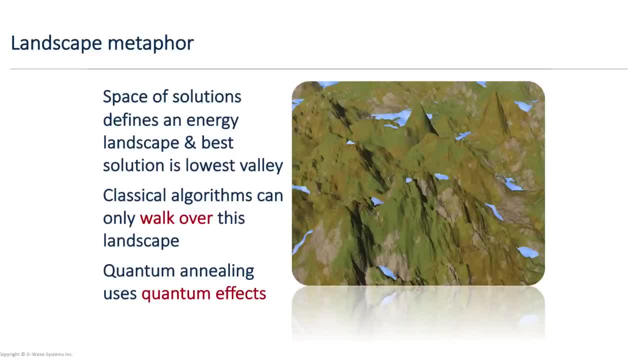 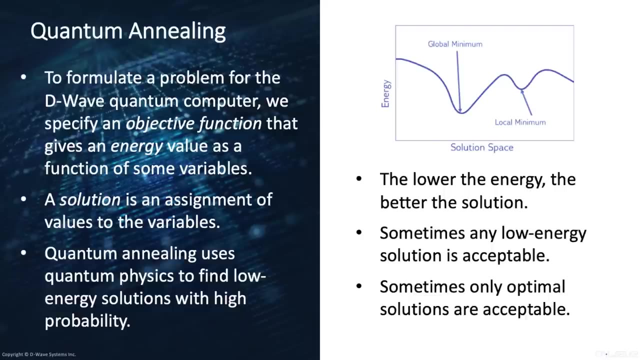 looking for lowest energy states as a function of the problems variables. In other words, where is the minimum? How do we find that? And so let's sum up what we've talked about here In order to formulate a problem for the D-Wave quantum computer. 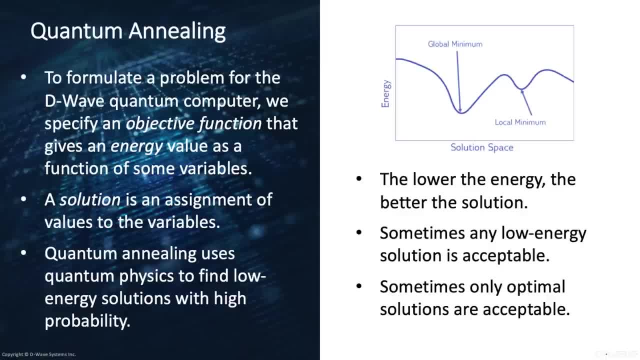 we're going to specify an objective function that gives an energy value as a function of some variables. So in other words, there's that mountain peak on the right, only in the right. of course it's just shown in one dimension, But the global minimum is shown there. 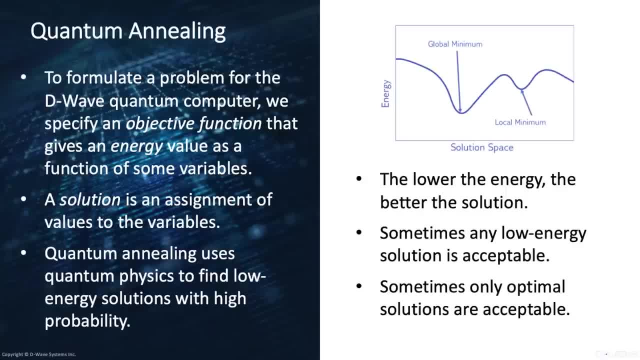 at the bottom and you express your problem in terms of those Q variables that I described. and a solution is an assignment of values And in the quantum computer we basically have a choice of either up or down for each qubit variable. There's no other choices. 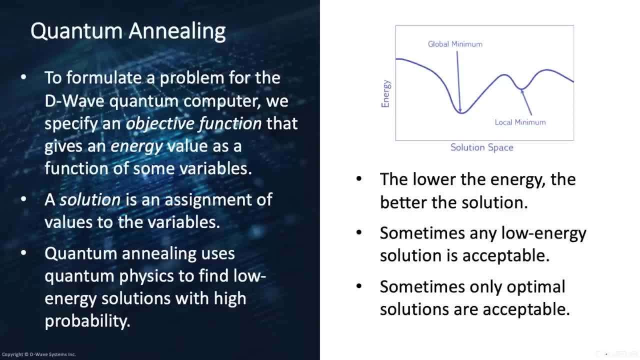 They're binary variables: up or down. corresponding could be to up spin or down spin. Quantum annealing uses the physics- and we've talked about this in the analog to classical annealing and so on. Try to find the lowest energy state with high probability, so that the system 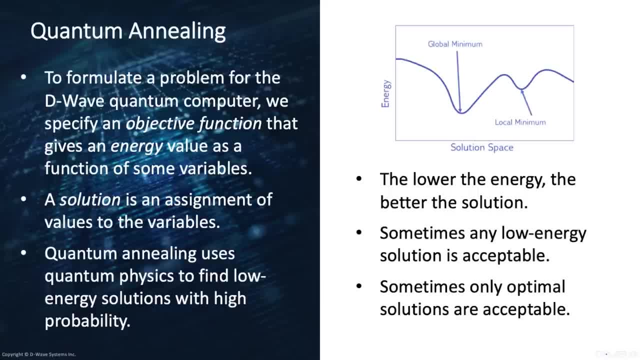 ends up in it, And we're going to talk a little bit as we go about how sometimes you only want the absolute lowest energy and sometimes energies which are very close to optimal are okay. And to motivate that a little bit, think about a UPS driver. 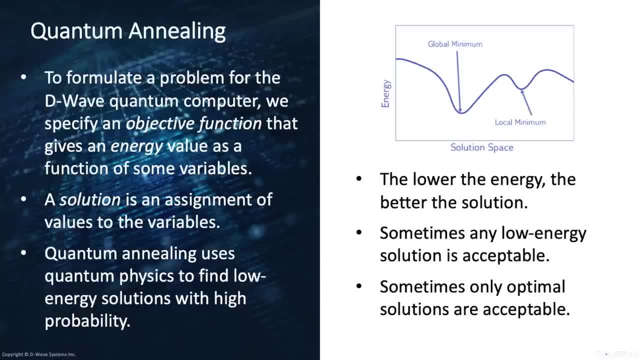 or an Amazon driver during the course of a day running what's called the traveling salesman problem, trying to hit a certain number of houses in a day. The solutions don't have to be exactly the lowest, because solutions that are only a few minutes off are not really going to be. 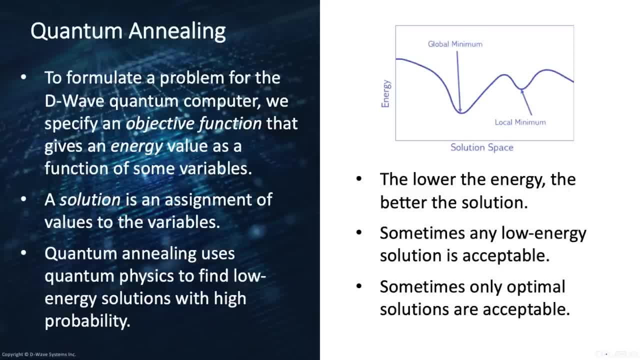 a problem for that driver, Whereas there are other problems where you absolutely want the minimum, And so keep this in the back of your mind. This is our goal: It's to find that minimum solution. So let's return also, though, to the D-Wave story. 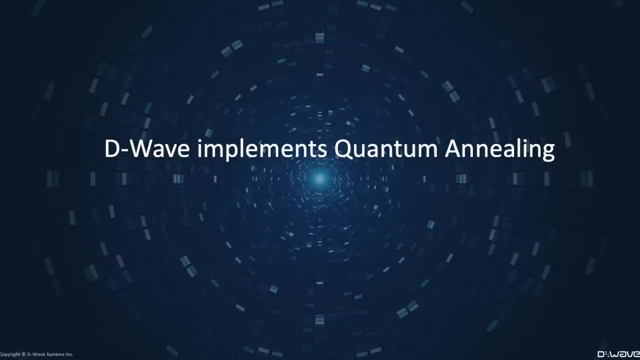 At this point, when D-Wave started out, it was basically collecting patents. You had a number of physicists working together on this technology, and the Katawaki and Nishimori papers, along with the Farhi paper, suggested a route forward, And so D-Wave decided. 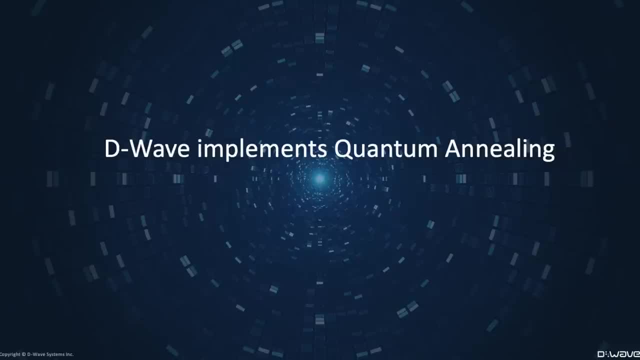 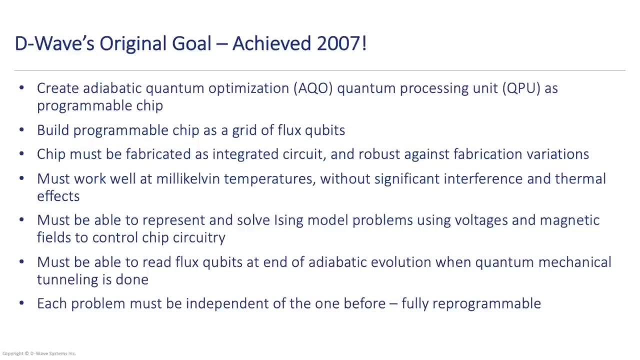 to try to build a machine to implement quantum annealing, to build a quantum computer. So D-Wave's goal, which was achieved, we'll talk about it in just a split second here- create a chip- basically it's programmable- that can do this adiabatic quantum optimization. 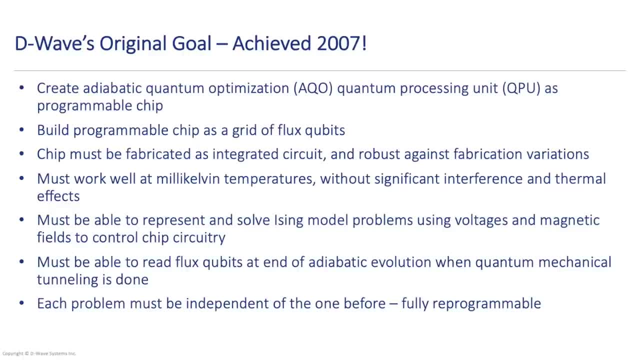 and build it as a grid of flux, qubits, qubits standing for quantum bit, which can either be one or zero, up or down. I should say one or zero, I should just say one, or I should just say up or down. in a moment I'll explain why. 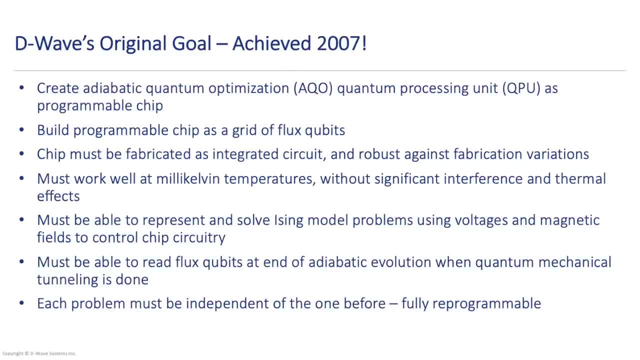 Fabricate it and also make sure that it's robust against fabrication issues, variations. Make sure it works at millikelvin temperature. be able to isolate it, be able to solve easing model problems using voltages and magnetic fields to control it. You have to be able. 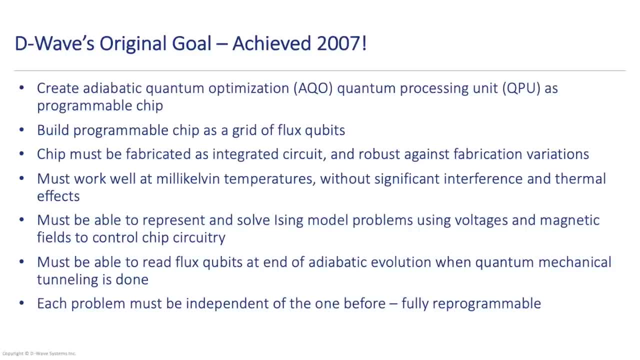 to read the flux qubits at the end of the cycle, those ones and zeros, or those ups and downs, or minus ones and ones, whatever they are- we'll talk about that later, when the quantum mechanical tunneling is all done. and to me the most critical is: 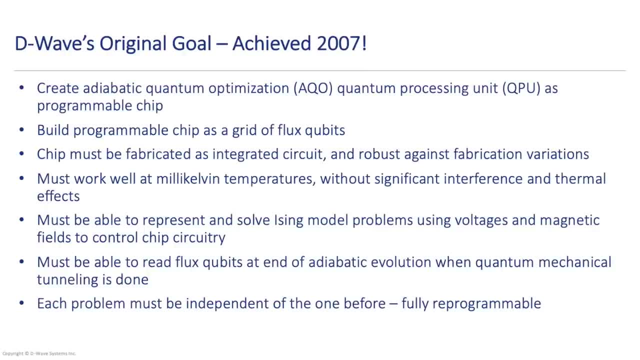 each problem has to be independent of the one before. it, has to be reprogrammable so that one user does not see the problems of another user, and D-Way was able to do this. as I mentioned, the first machine came out in 2008. 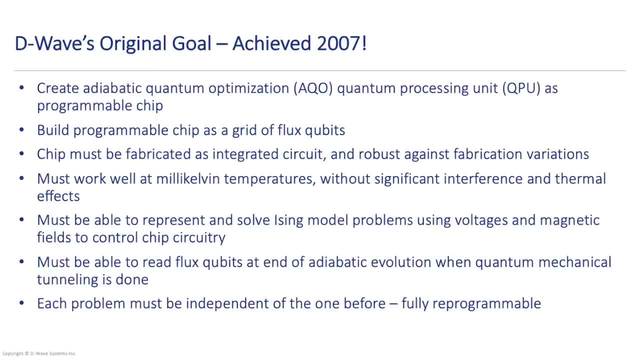 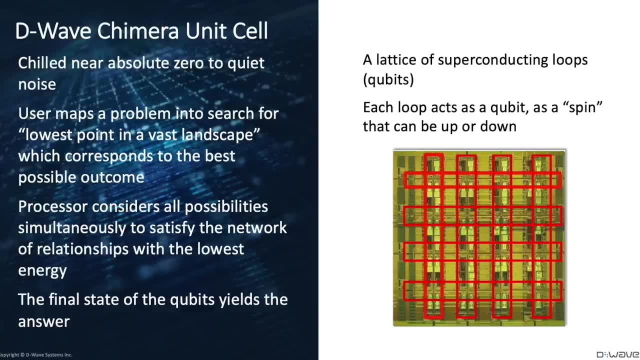 came out in 2007, and now let's dive in to the next bit of that. And so the unit cell in a quantum computer that D-Way built is called Chimera, and basically this slide goes over a lot of the things that we've talked about. 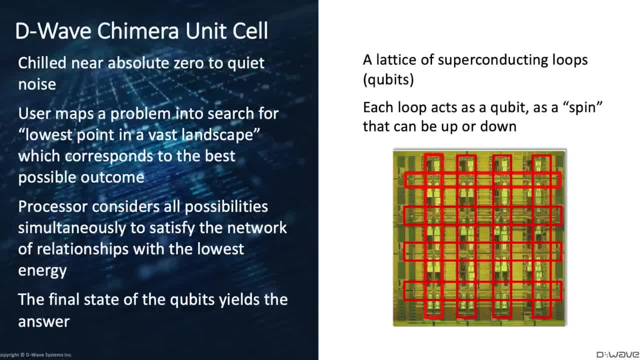 but you basically on the right side, is what I want to call your attention to. you build a lattice of superconducting lines or loops, and D-Way chose to implement its qubits as superconducting metal wire loops, and you may be familiar with some other ways. 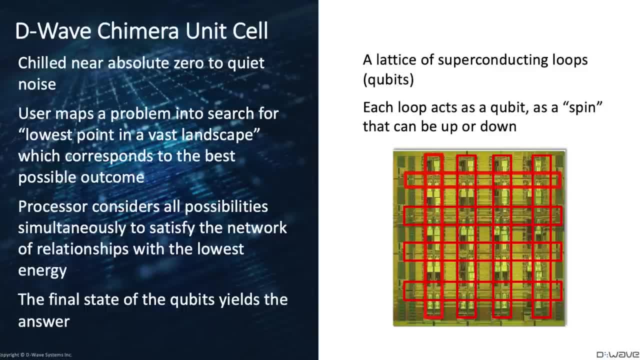 to create the qubits, ion traps being one that's also popular. this was one way to do it and each loop acts as a qubit with a spin that can be up or down and the unit cell in the Chimera architecture. on the D-Way of 2008. 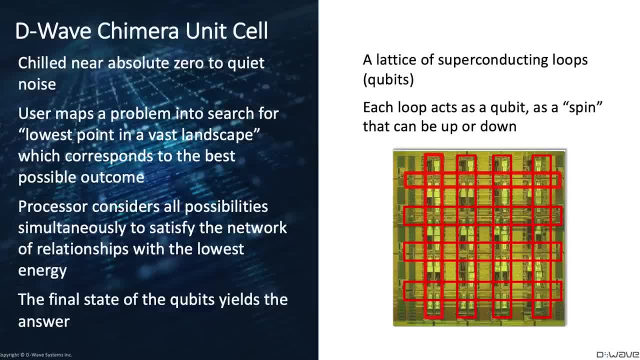 or on the D-Way of 2000q. looks like a 4x4 grid like that, where there's actually 8 qubits in each unit cell and 16 couplers. the couplers where the loops interact are connectors between those qubits. 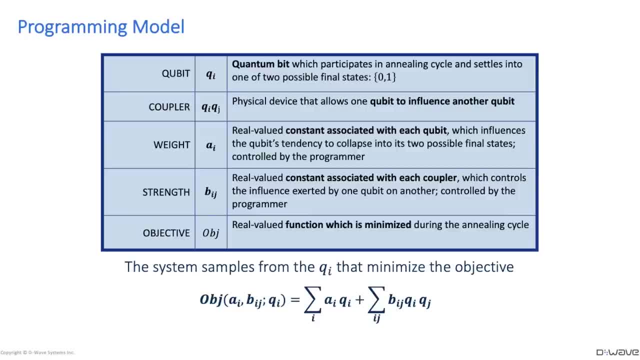 which we're going to talk about in just a moment here. And so, finally, we arrive at the programming model itself. You've got the sum at the bottom of the screen and the numbers, the little a's, and there's one for each qubit in the system. 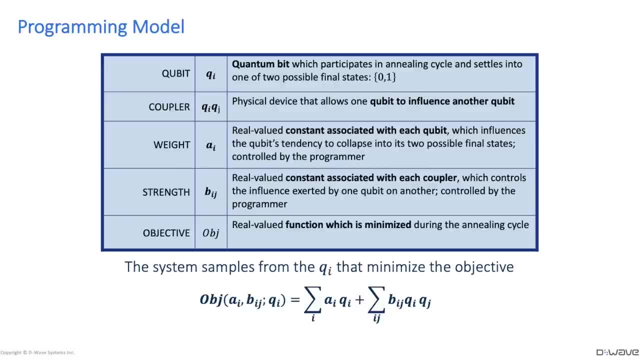 are called biases or weights, and the numbers b, the b? i j's are called couplers or strengths. and so the programmers goal, basically, is to set the a? i and the b? i j's so that when the machine calculates the objective function, it finds the lowest energy. 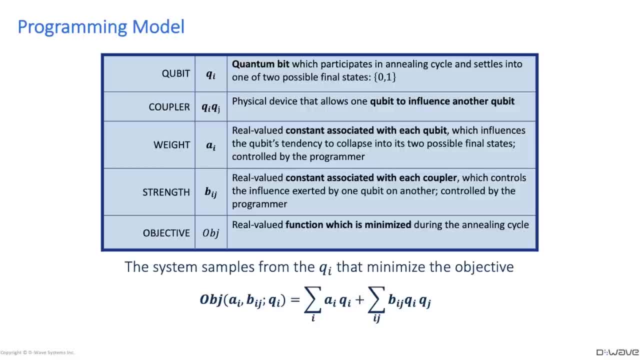 with a particular qubit solution and, according to the way we've set the a's and the b's, we're hoping to influence the machine to find the lowest solution that we can get in this what is called objective function. So hopefully you've got this sense. 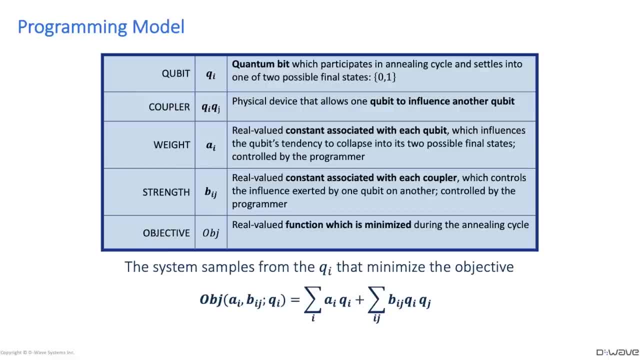 of what these are. we're going to learn how to set the a's and b's. we're going to do that in a particular way that'll lead us to the lowest energy solution when the annealing cycle runs. Now it turns out that this problem 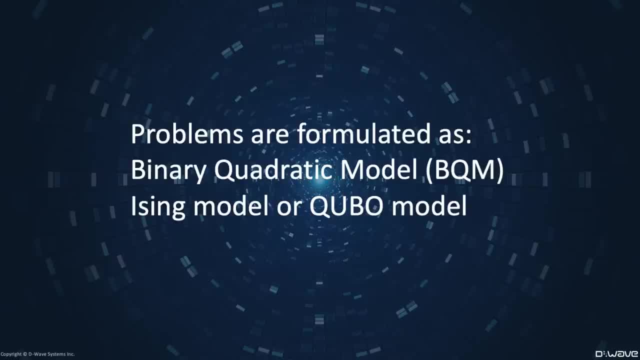 with these a's and b's and the q variables was well known to mathematicians and operations research scientists. and basically, there have been two ways to formulate the problems that you're going to solve with this computer, and one is called the Easing Model, which I'm going to talk about shortly. 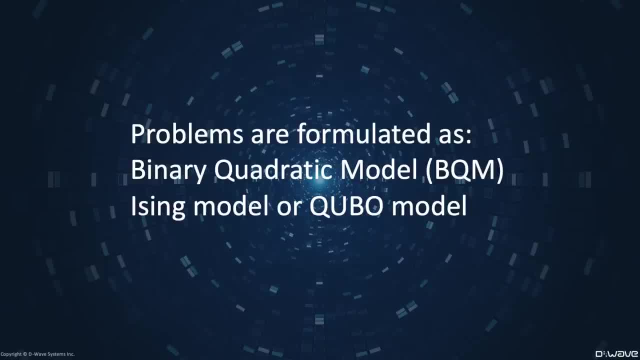 and the other is QUBO- Quadratic- Unconstrained Binary Optimization, and they're both perfectly good ways to do it. there are advantages to both, which I'll talk about. each one has its own, but they're basically unified in what is called a Binary Quadratic Model. 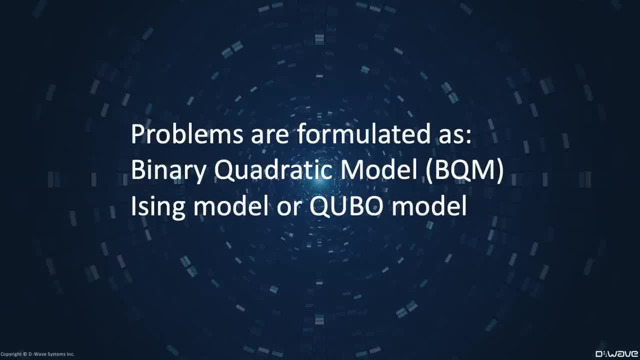 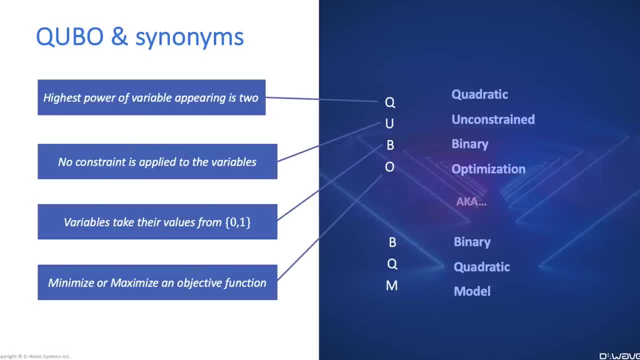 which is a. that's a D-Wave term but it's a useful one that will cover both Easing and QUBO, and the reason for the name QUBO is that quadratic for highest power of the variable appearing is 2. no constraint is formally applied. 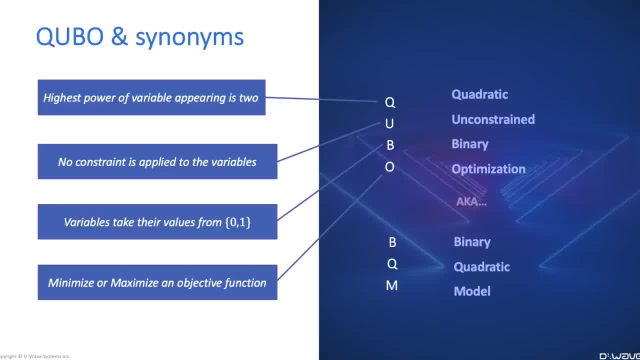 to the variables. that's the unconstrained part. the variables take their values from 0 and 1. that's binary, and you're going to minimize or maximize some objective function like the one we talked about. that's the O for optimization. so QUBO stands for 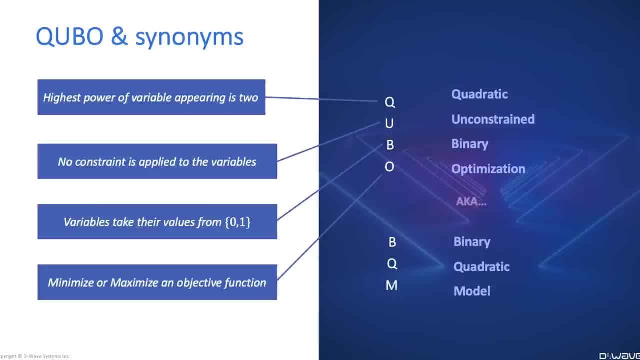 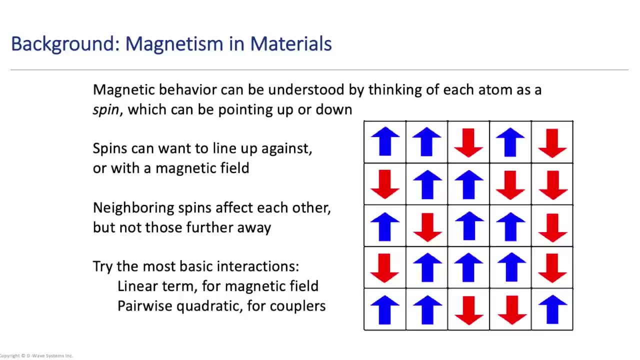 Quadratic, Unconstrained Binary Optimization. and now I'm going to give you a little bit of a sense, physically, of where these models came from, because you might be wondering: where did this Easing Model come from? and this happens to be: take yourself back to the early days. 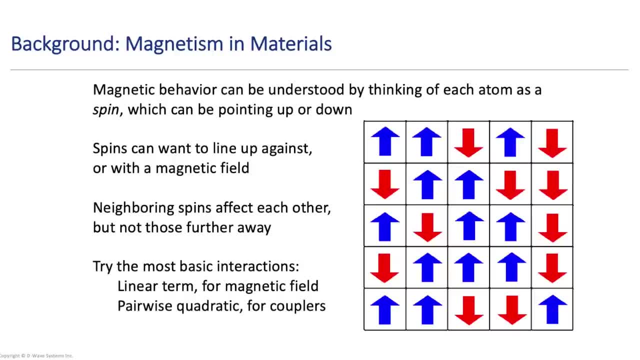 of the 20th century, people wanted to know why certain materials showed magnetic behavior but others didn't. some metals could be magnetized readily and kept their magnetism. other materials couldn't, and a way to model it that's very simple- is to think of each. 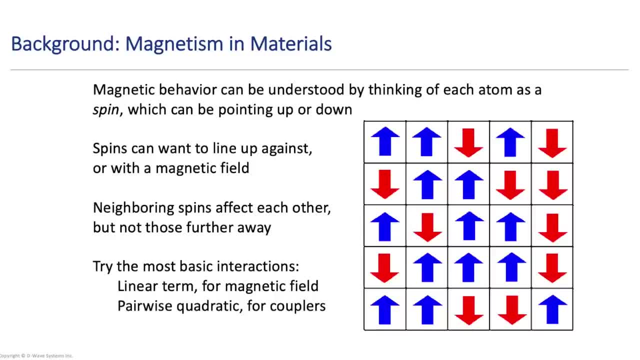 each atom as a spin, something that can either point up or down and the spins want to line up against or with a magnetic field. and if, if we think about it in a simple way, that neighboring spins can affect each other, the ones next to each other, or under or above? 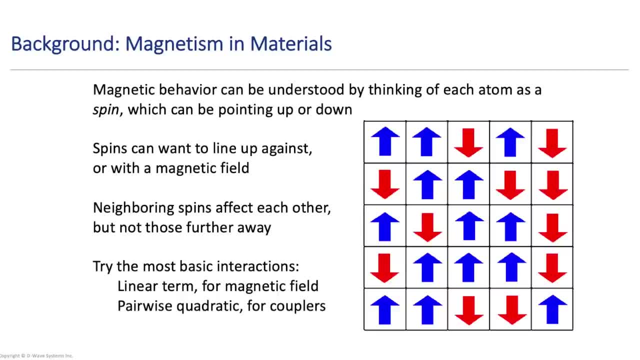 but not those farther away, and we try the most basic interactions. in other words, assume that they influence each other in some linear, very simple way. in other words, picture a spring being pulled back. if you pull it more, it'll push, pull back with more force, but in a linear way. 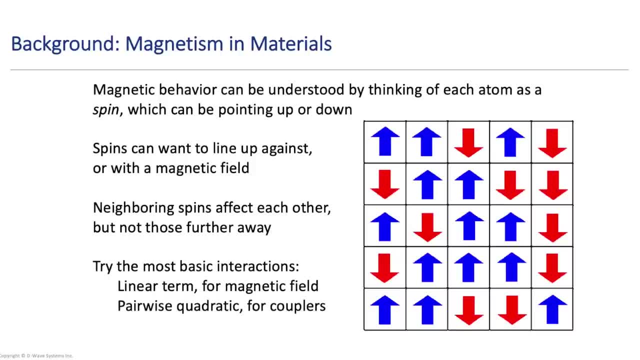 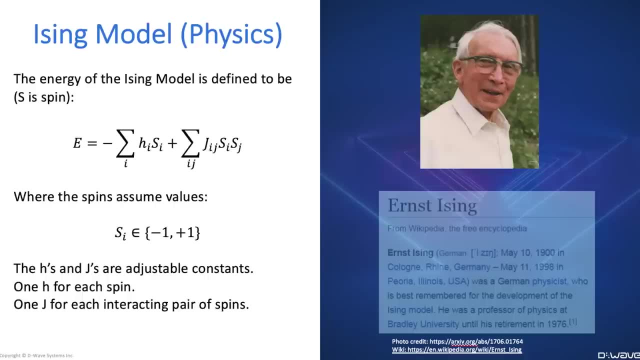 and pairwise quadratic only for couplers, and it turns out that this is indeed now known as the Easing model, and here's the reason why. Ernst Easing was a graduate student in Germany, and he was given the problem of one dimension: coming up with a magnetism model. 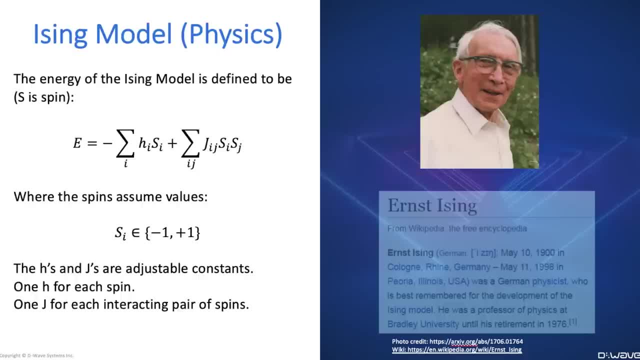 and he basically gave him this model, which did pretty well and eventually was extended to two dimensions in the 1940s. but the main point is that what is now known as the Easing model looks like this: you have a negative sign which is different than cubo. 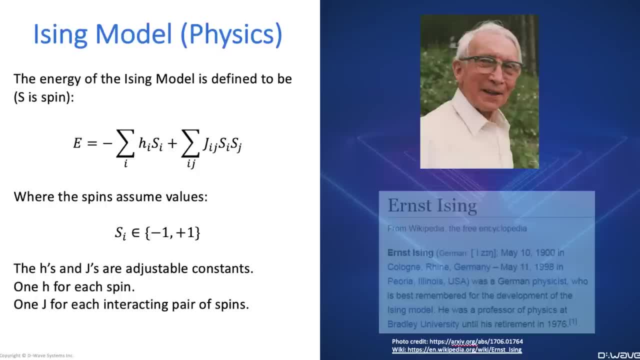 with numbers that are referred to as h's and j's instead of a's and b's, but you can recognize the terms there: the s sub i's instead of q sub i's, and s i s j instead of q i, q j's and in the Easing model, 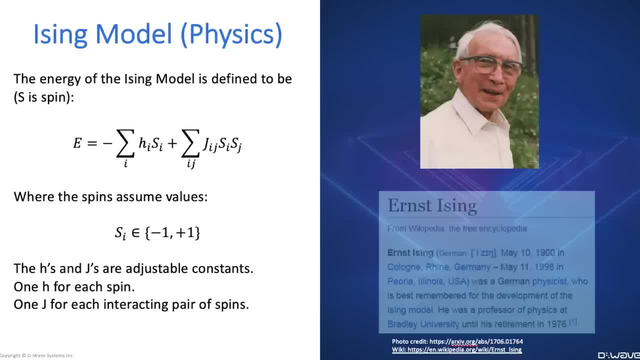 it's minus one and one there in the middle of the page, instead of zero and one, and we're going to focus on cubo. but my main point is that both Easing model and cubo are both perfectly valid ways to formulate a problem, and just for interest. 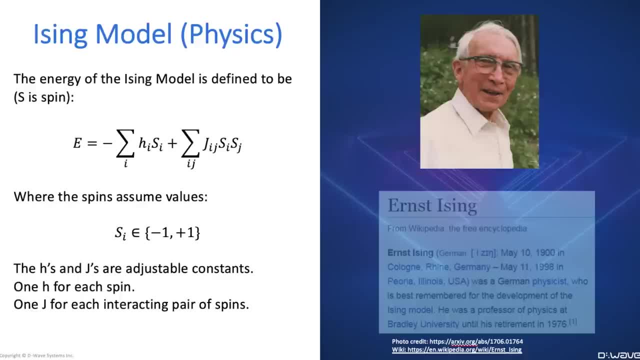 Easing lived a very long life. he was 98 years old when he passed. he was a professor in the US for a long time and there's a picture of him later in life. here's a direct comparison between the two. you can see at the bottom. 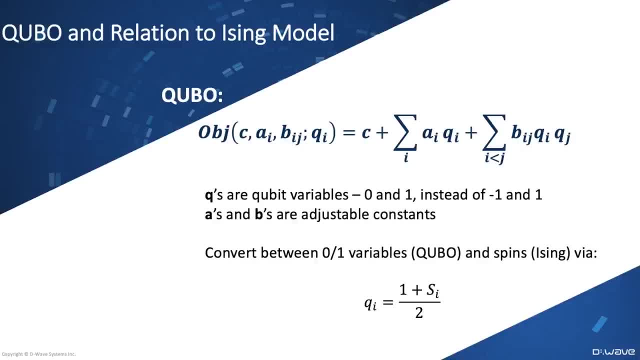 that a single variable substitution will transform one into the other, and the cubo model is in the middle of the screen there. but what I meant is that we can basically use either one. physics and physicists tend to like the Easing model better, whereas mathematicians and 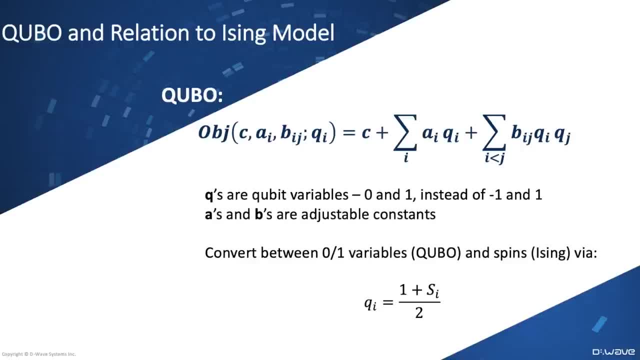 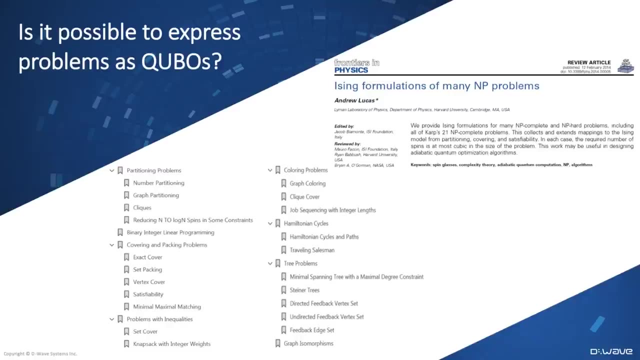 people, like in operations, research and so on, tend to use cubos, but you'll be able to find both, and so another question is, if this is so well known, what problems have been solved with this before, and this paper by Andrew Lucas appeared in 2013-14. 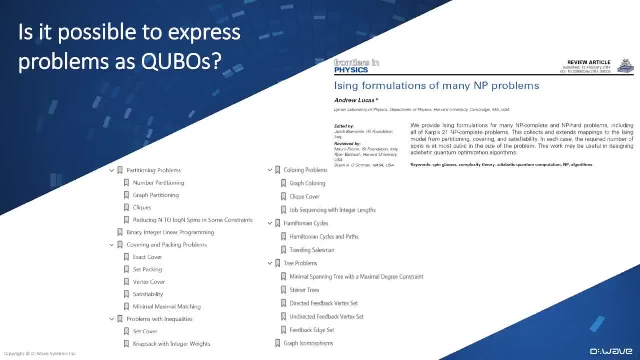 where he basically works through many famous NP-hard problems. NP-hard a term in mathematics that isn't important to define for us here, but many of these problems are very well known as very difficult to solve. easy to check the solution, but difficult to solve. traveling salesman is one of them. 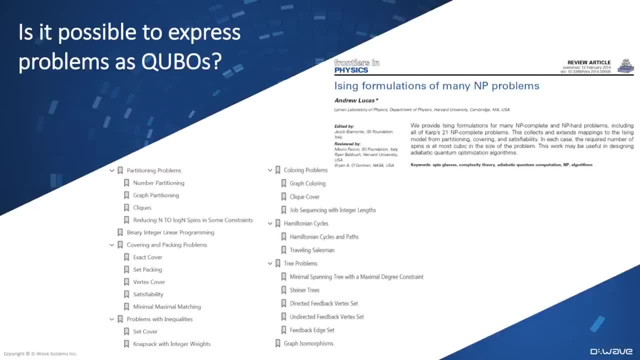 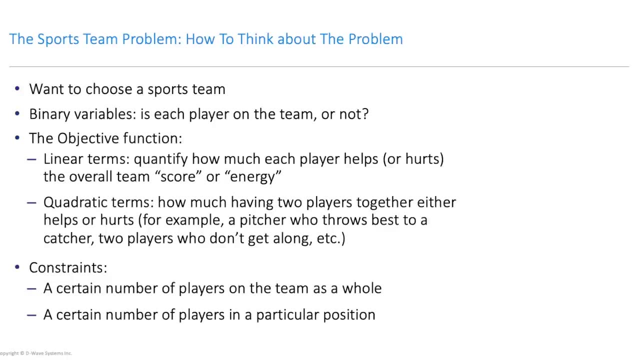 so I highly recommend you seek out this paper if you're interested in some of the problems that have been solved with cubo. so before we leave behind this abstract stuff and get into more specific problems, think about a sports team as an example of a model like this. 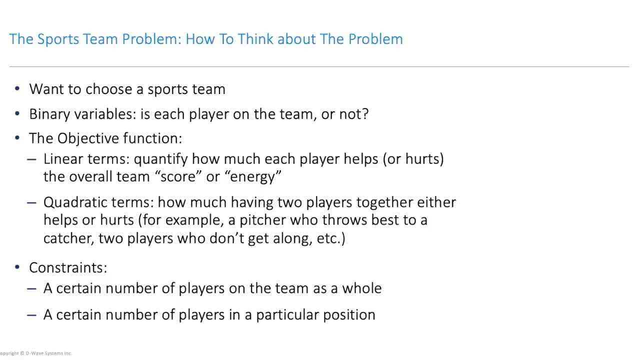 there's an objective function telling you sort of how good the team is, some number and there's linear terms quantify how much each player by him or herself helps the team, depending on whether he or she lowers the energy or raises it, and quadratic terms are pairwise teams that have players. 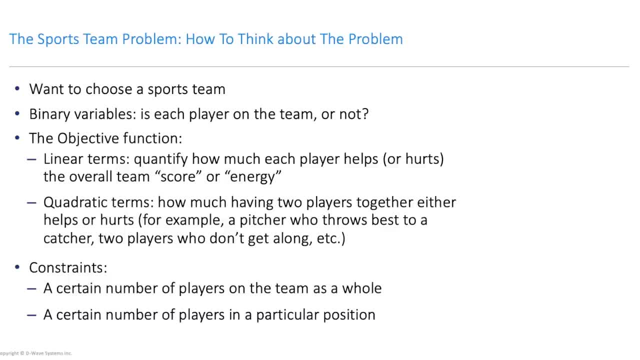 who play together well or in some cases do not actually- and then the objective function will be something like that. and then you have constraints where you're only allowed a certain number of players on the team or a certain number of players in a particular position, like hockey, for example. 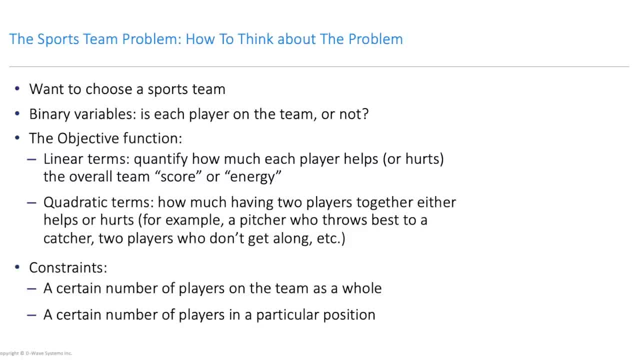 only a certain number of goalies usually are on the roster, so this is another problem that probably would respond really well. we've done some team picking of small teams, but I suppose someday, when the computers get big enough, we'll have NFL Draft being done with quantum computers. 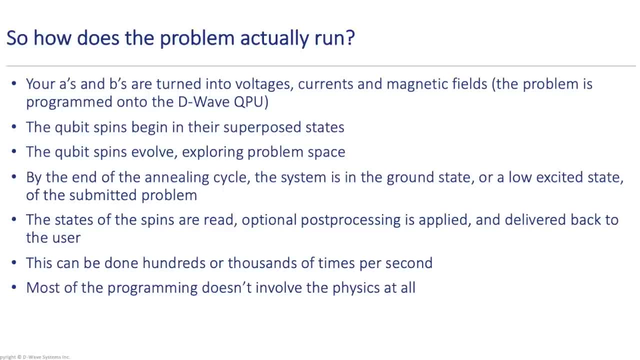 and before we go on, let's summarize how all this works. how does the problem actually run? the answer is: your A's and B's get turned into voltages, currents and magnetic fields. the qubit spins begin in their superposed states and they evolve, exploring the problem space. 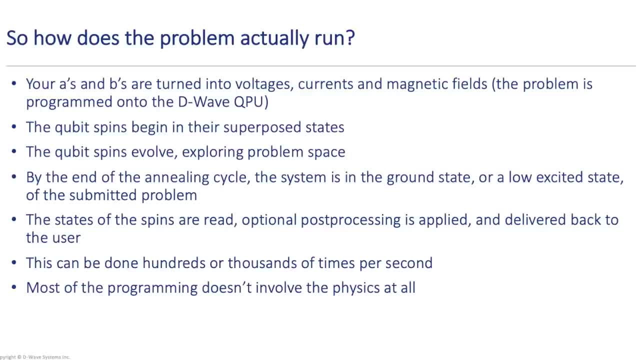 and by the end of the cycle, if all is good, the system is in the ground state or a low excited state of the submitted problem. you read the states of the spins, you apply post processing if you want and you deliver it back to the user and this can be done. 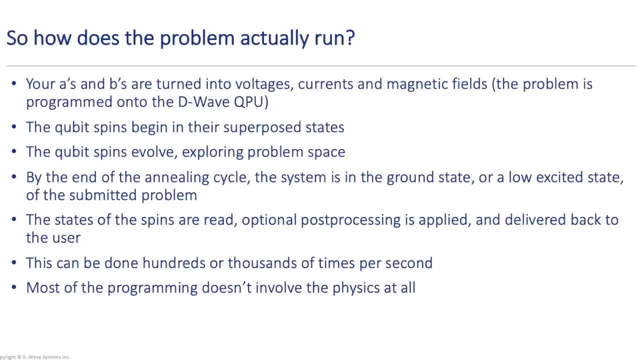 hundreds or thousands of times per second, and you don't really need to know the physics in order to get started. anyway, there's dynamics within qubits, between qubits and each other, but we don't really have to worry about all the work that was done to formulate this. 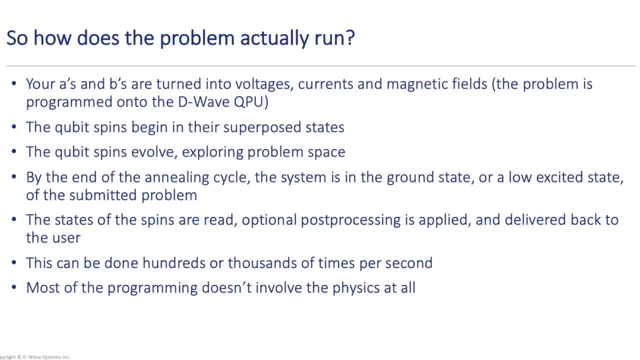 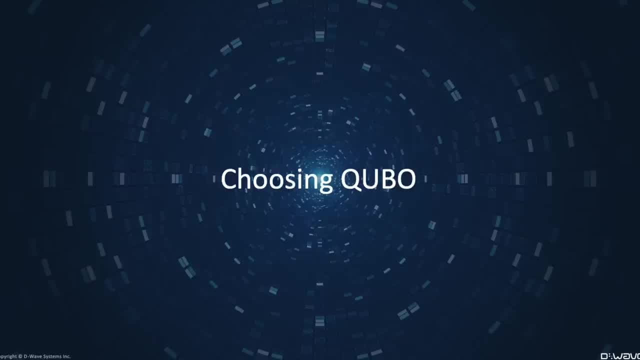 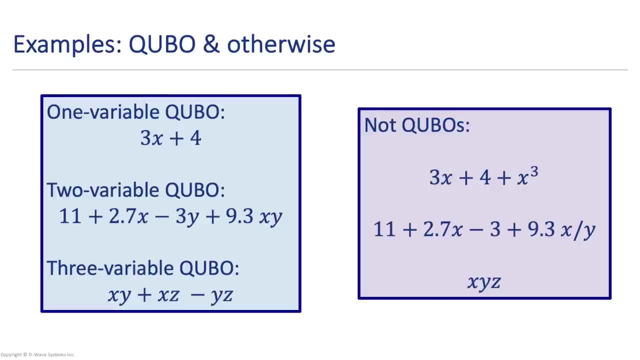 it's kind of out of the problem by this point. so let's go forward now and focus on some cubos, learning what they look like, and then setting up a problem looking on the left, as we mentioned, linear and pairwise quadratic only. so 3x plus 4 is ok. 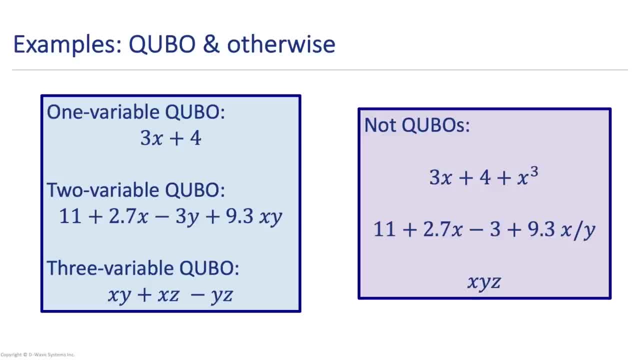 the middle one with the x term and the y term and x times y. that's ok. finally, at the bottom, a three variable cubo involving pairs of those variables: x, y, xz and yz. what is not ok is on the right things like x cubed. 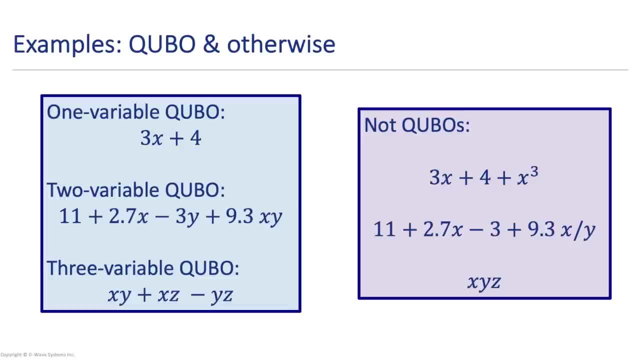 or x divided by y, or a triple product: x, y, z. now, if you're familiar with this from before, you know that there are algebraic ways to get rid of things like x, cubed and higher order terms, but that's out of our scope here. 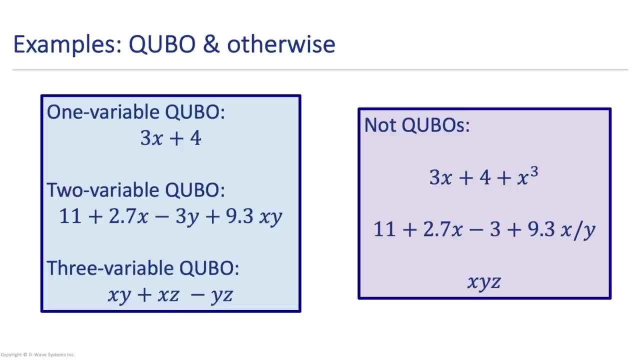 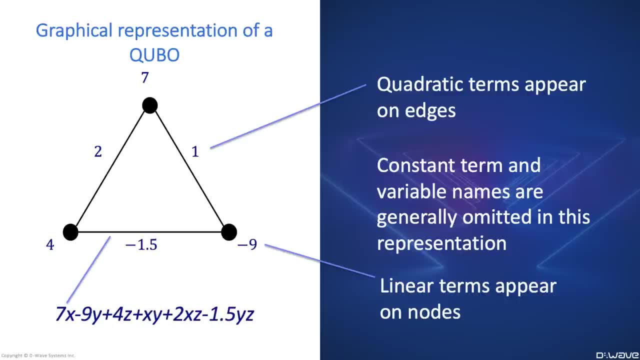 we're going to focus on the linear and quadratic terms. we won't worry about algebraic reductions and things like that. and here's a graphical way to look at a cubo. the quadratic terms appear on the edges: the one, two and minus one and a half. 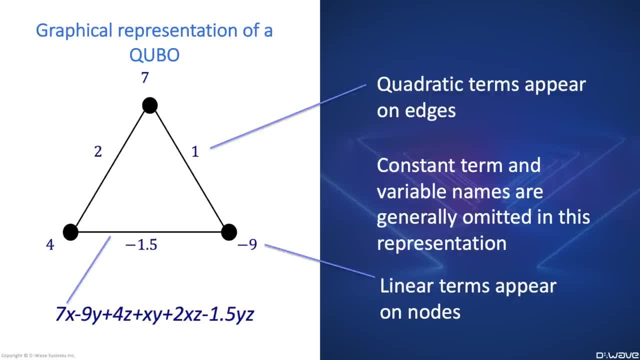 the the linear terms appear on the vertices or nodes, like the four and the minus nine and the seven, and so at the bottom here you can see the cubo that we've chosen, and constant terms and variable names do not appear on the graph. we'll come back to that constant. 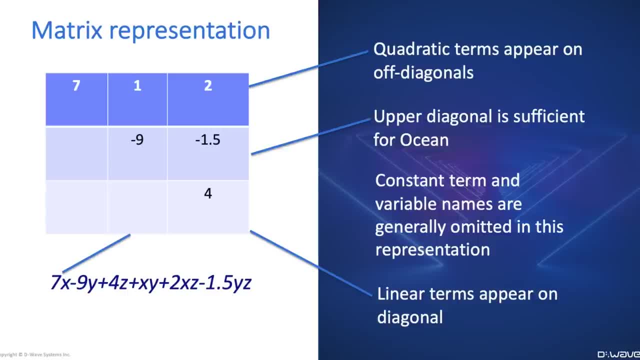 later on- and here's another way to represent a cubo, and it's the same one from the previous slide- you put the diagonal terms as the linear coefficients seven minus nine and four, and the off diagonals represent the couplers or the off diagonal terms, and so you can see that. 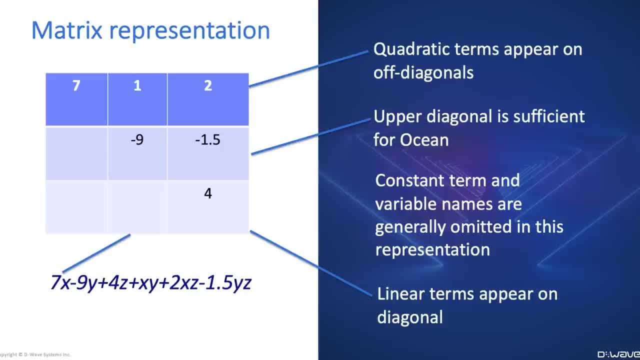 one times xy is up there in the one comma two position, and two is in the one comma three position, and so forth. why are they on the diagonal? it's because- and this is an interesting thing- in cubo, x squared equals x. in other words, if you think about it, 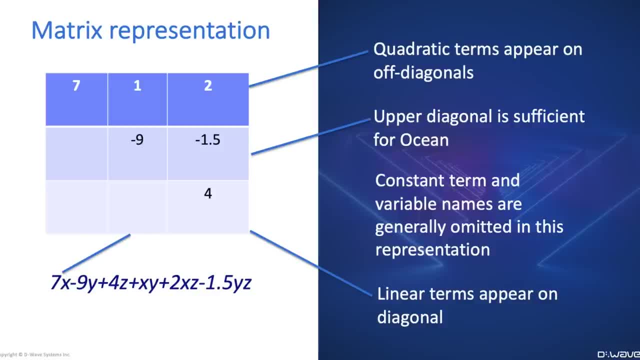 zero squared equals zero and one squared equals one. so it's okay in this case that x squared equals x and we're able to put those on the diagonal of a matrix. and this is one of the advantages of why cubo is a little bit, maybe simpler in some problems. 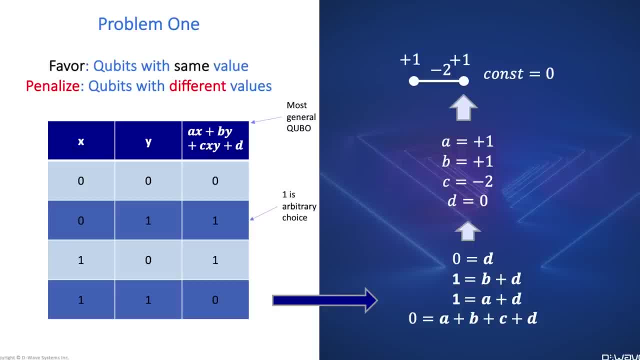 algebraically. and finally, here's our first problem. let's just call it problem one. the goal is that I want to run a two qubit problem on the quantum computer, such that the result will be that I get two qubits with the same value coming back. 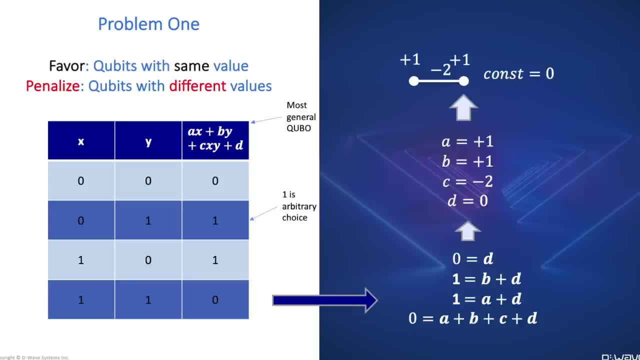 and that I do not get solutions of the form qubits with different values. now, with only two qubits, we have four possibilities, so we make a truth table here. you can see them: zero, zero, zero, one, one, zero and one one, and so I'm going to do some algebra here now. 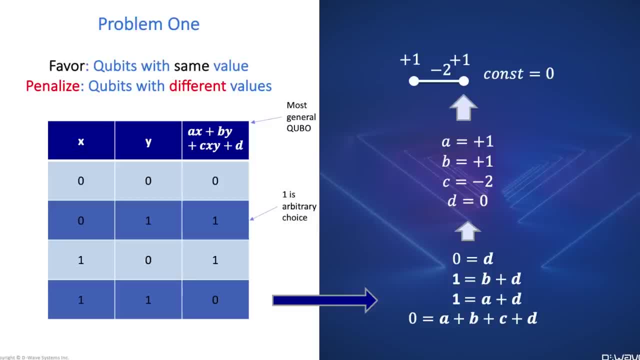 and show you why we pick a and b and c and d- and that's the same as the a's and b's, just different letters- to represent the solution to this problem. the most general cubo that I can have is in the box there, so I'm going to take 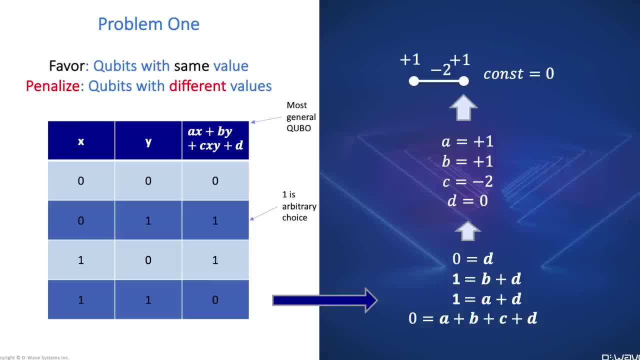 x plus by, plus cxy plus d. there's no other terms, and what I just simply do is I take x and y and I put them in, and there's what happens in the third column. zero and zero have to be on the first row and the fourth row. 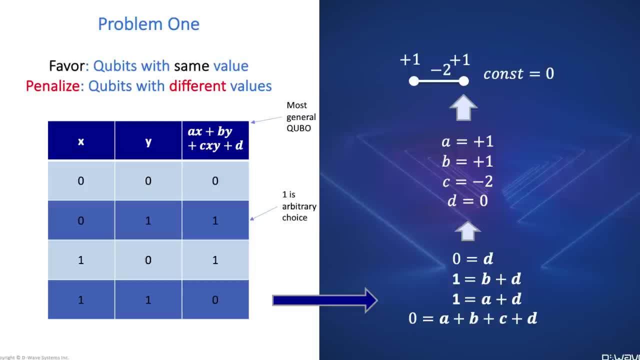 and I want one to be on the second and third, so that lower energy is found for the qubits, which are the same, in other words the zero, zero solution and the one one solution. I want those to be lower, so I'm going to insist now. one is an arbitrary choice. 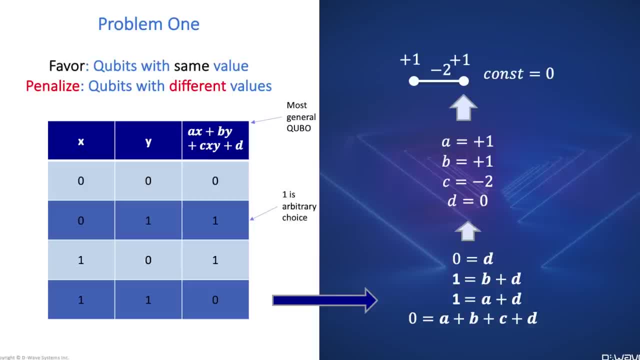 could be six, could be five, whatever, but in this case it's just it's higher than the other. that's the main point. if I go over and do the algebra to the right there, I learn that d is zero. the solution that I come up with is that a and b have to be one. 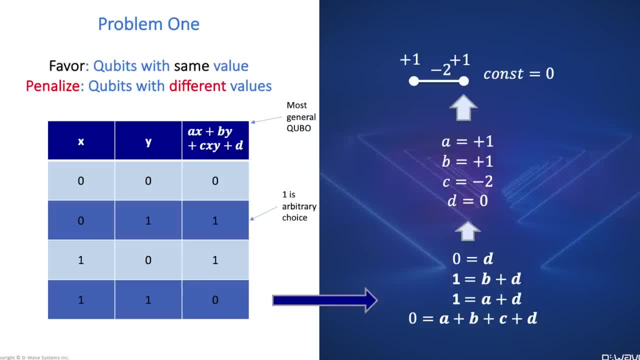 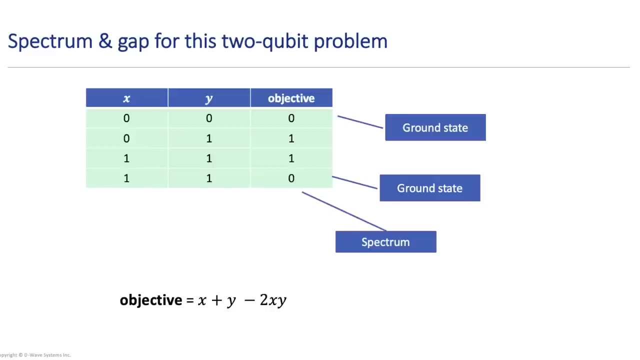 and c has to be minus two and d is zero. there's no constant in this case. I call it the one one minus two solution. and so now let's look at what this cubo does when we run it. so the cubo for this is just. 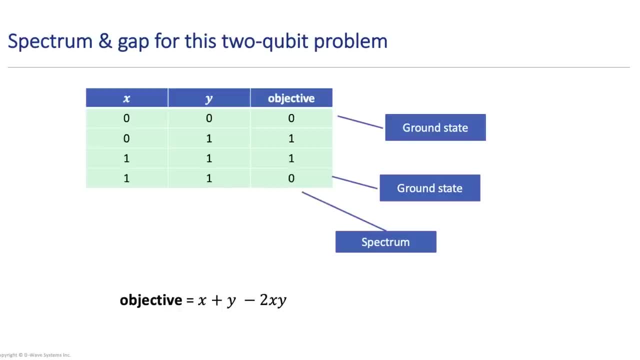 x plus y minus two, xy. that's the one one minus two solution we just talked about. and when you run it- and I'm not showing you how to run it yet, but you can see it's called the spectrum. the results. the first and fourth rows featuring the zero: zero. 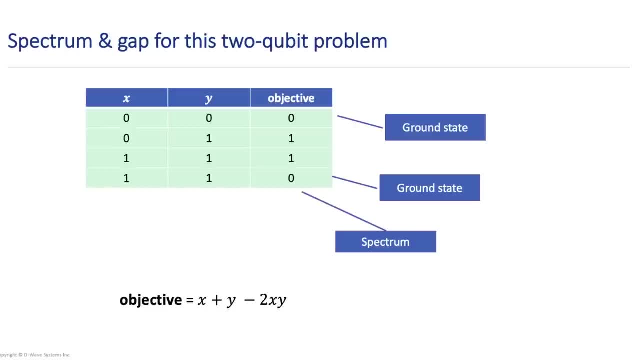 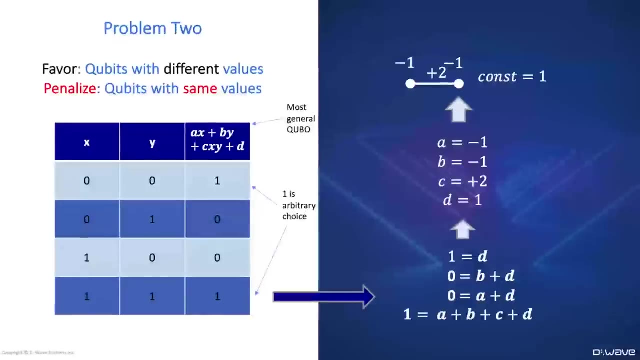 and the one one. solutions are indeed the lowest energy, that is called the ground state, and then the middle rows, one and one, are higher energies, or excited states. so let's move on now to problem two, and in problem two I want to favor the solutions with different values. 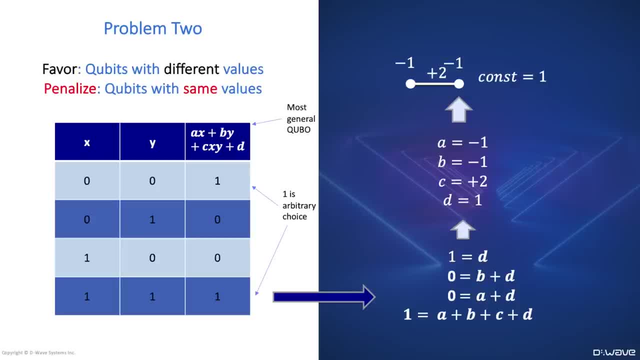 in other words, I want the middle rows- this time zero, one and one zero- to come out lower, and so I'm going to put the value of one on the higher solutions- the zero, zero and the one one in this case. and we work through the algebra and different things happen. 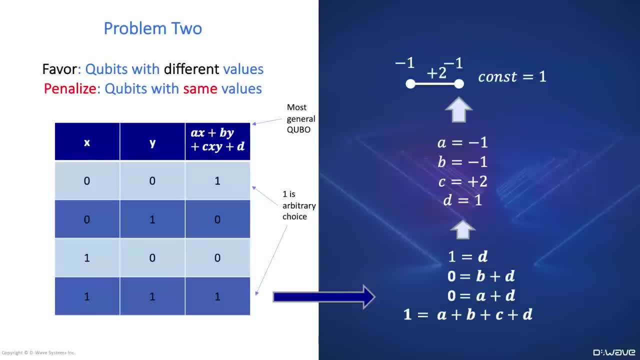 this time. instead we get the solution to be a and b are minus one and c is two, and then there's a constant of one. and it sort of makes sense, because earlier we had the solution one one minus two. you sort of think of it: these are favoring the opposite one. 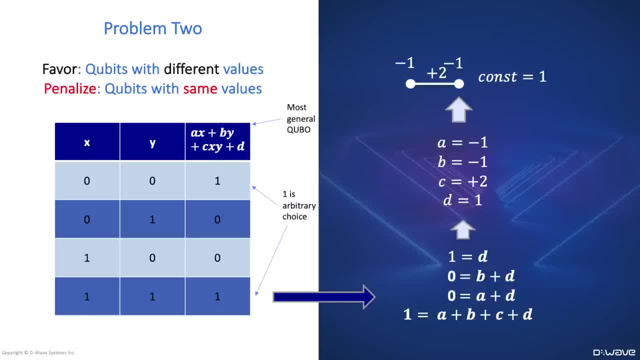 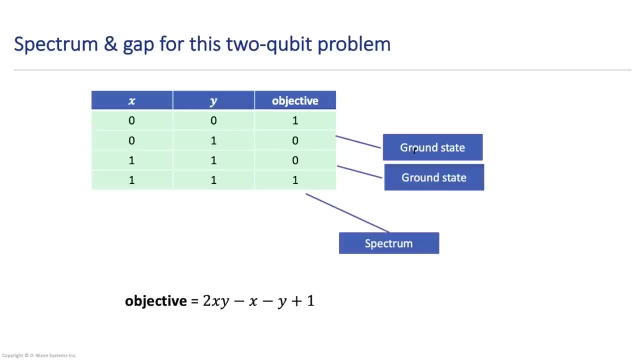 so it sort of makes sense that the minus sign should do that. so let's have a look at the spectrum. and this spectrum shows that, as we expected, the fourth and first rows come out with higher energy. this time they're excited states. the middle rows are the lower. 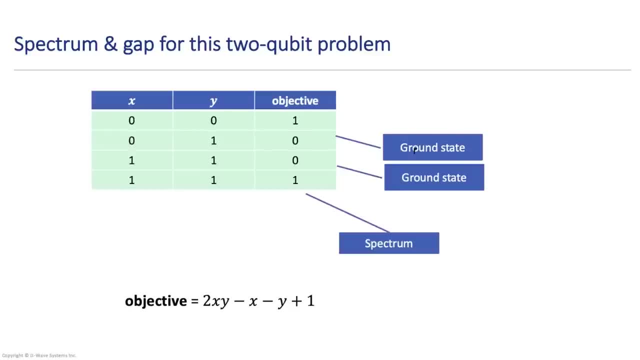 energy, the ground states. there are two ground states with the same energy and in this case the objective is two x y minus x minus y plus one, where one is a constant in this case, and the reason the constant is there is: we want to end up with the same energies. 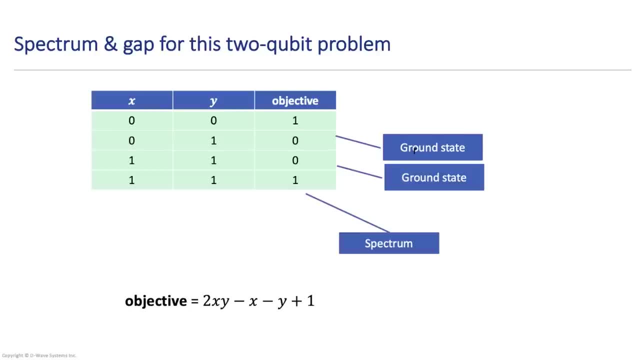 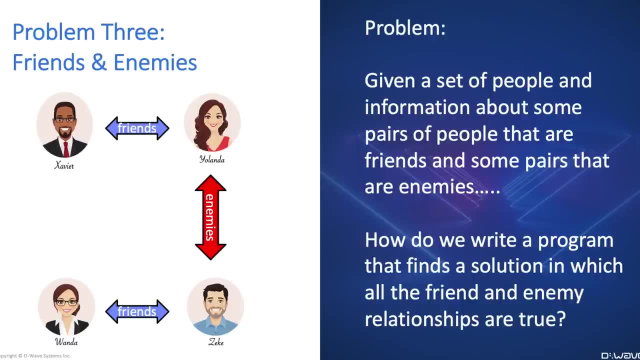 as in the previous problem, that's what the algebra insists on. and now let's consider problem three, which will feature four individuals- Xavier, Yolanda, Zeke and Wanda, and they're going to have friend or enemy relationships. we want Xavier and Yolanda. 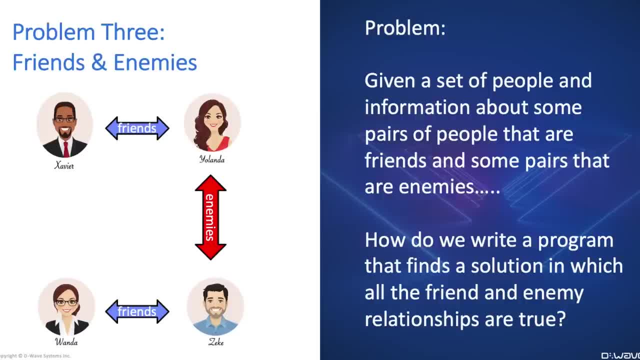 to be friends. we want Yolanda and Zeke to be enemies, and we want Zeke and Wanda to be friends. how do we write a program that finds a solution in which all the friend and enemy relationships are true? so the first question is: what does that mean? 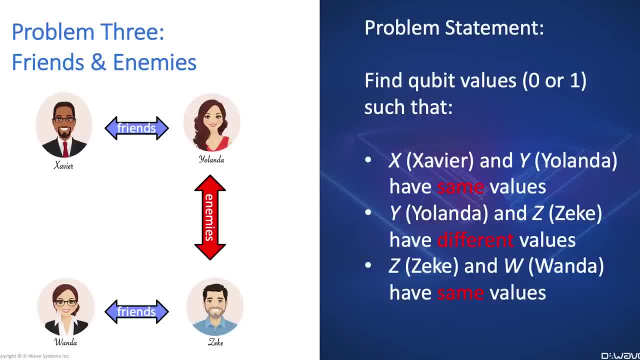 so another way to restate the problem is this: find qubit values, that is zero or one. we're in cubo such that x and y are qubit values because they're friends. Yolanda and Zeke have different values, that's y and z. 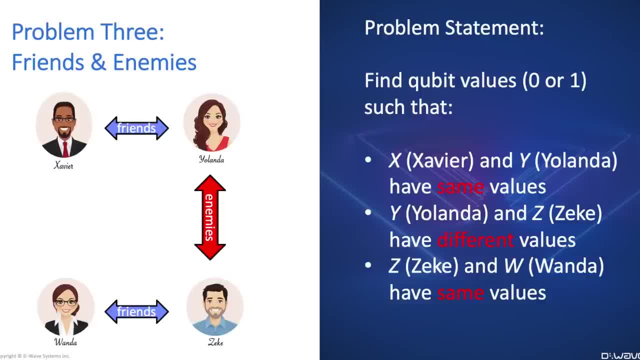 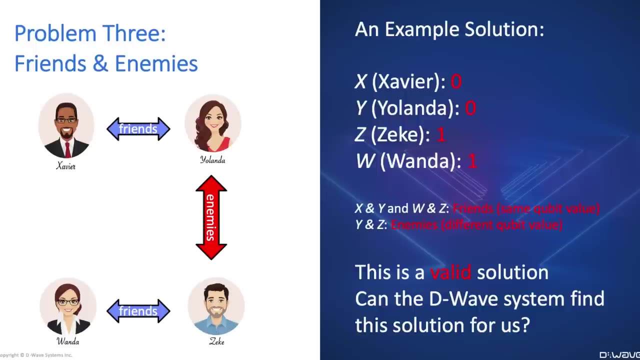 across the right side, and then Zeke and Wanda, z and w have the same values. so hopefully you can see what we want to do. we want to use the quantum computer to solve this simple problem. so in case it's not clear yet, let's look at what. 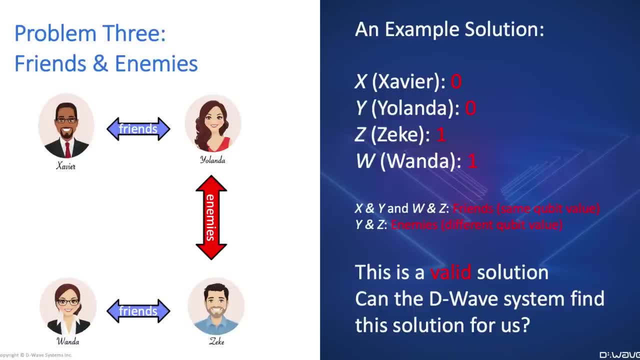 we can do. an example solution would be x and y having the value of zero- that's the same, so they're friends. y and z having the values zero and one respectively, so they're enemies, they're different. and then z and w having the same value, so they're friends. 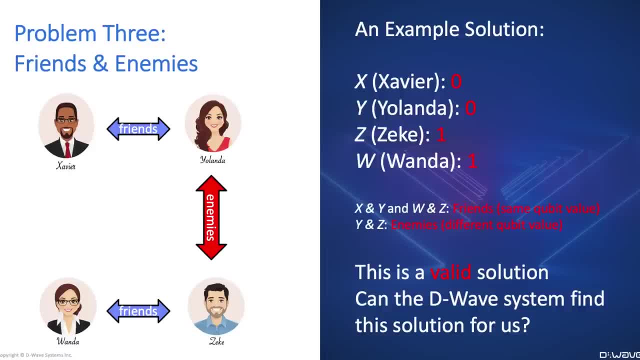 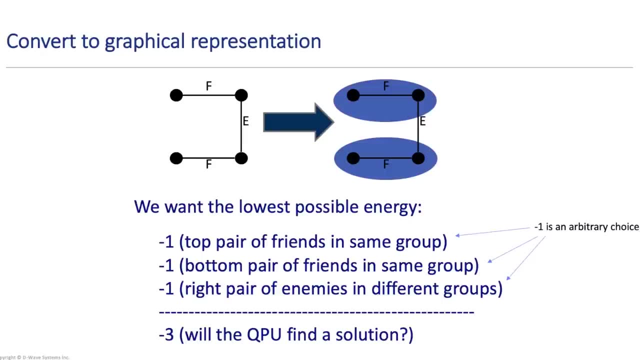 but the question is: can the d-wave find the same value for us? the first thing we do is to turn this into a graph, where we're going to look for a very simple graph with nodes across the top and on the right and on the bottom: friendly relationship. 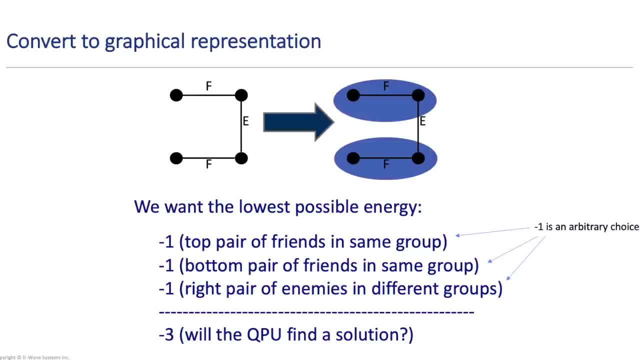 the bottom And we want the lowest possible energy that we can get, And so we're going to make a assumption here that for the top pair of friends I want the lowest energy to be minus one. I don't have to. In the example you saw earlier it was actually zero. So in this case we're going 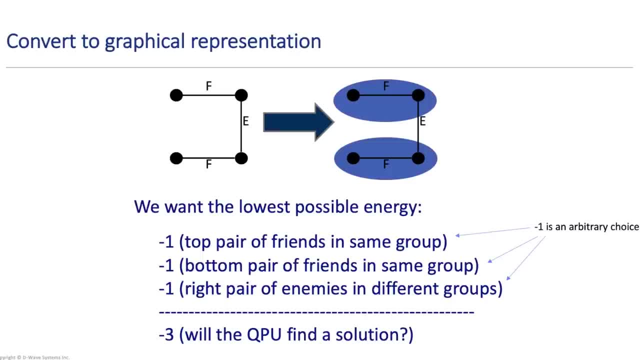 to make it minus one. We want the bottom pair of friends to have energy minus one if they're the same, And on the right we want the pair of enemies to have energy minus one if they're different. And again, the minus one is arbitrary. So the total lowest energy, lowest total energy. 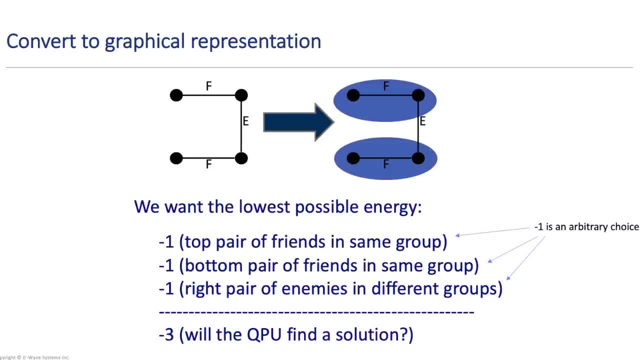 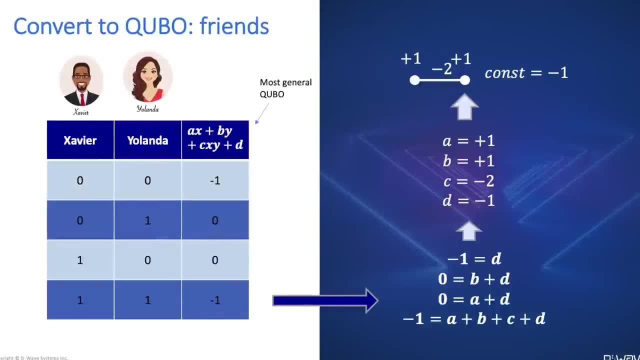 either way will be three, And so the question is: will the QPU, can the QPU find a solution to this? And so we're going to do the analysis that we did earlier in the unit a little bit different, As we'll see. In this case we'll put Xavier and Yolanda, X and Y across the top, with the most. 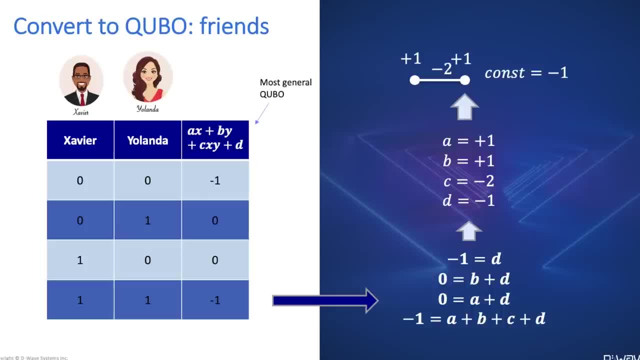 general QBO Again. this time, though, I want the lowest energy for the same qubits solutions to be minus one, and the higher energy for the different qubits to be zero, And so, if I work the algebra out, what I get when you get to the top of the right side is one one minus two Again. 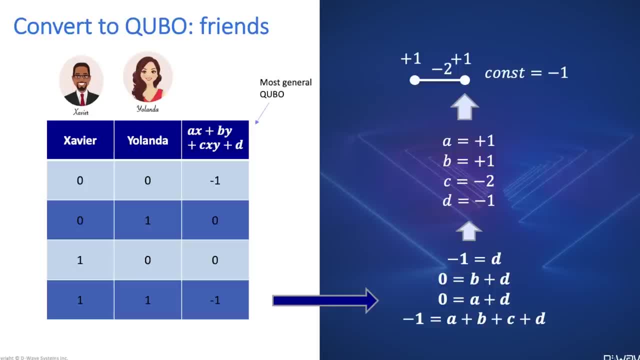 much like exactly like we got last time, but this time I've got to put a constant as minus one overall, And so that that constant is basically used to adjust the energies to where I want them to be. In this case, as I mentioned earlier, I want the friend relationships to have energy minus one. 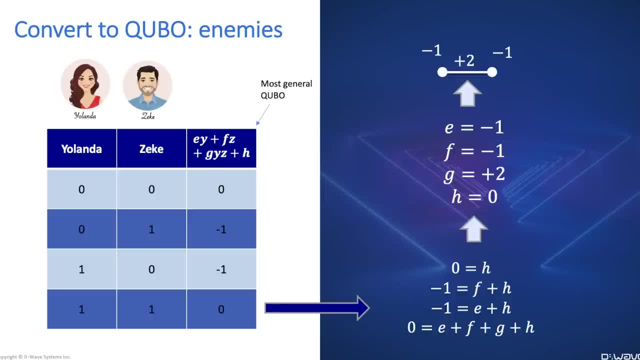 if they hold, Then for the enemy relationships, for Y and Z, notice it's the same thing in the table, except this time I want the middle two rows, the second and third rows to have energy minus one, and the first and fourth rows, the same qubit values, to have energy zero. And so, if I work the algebra out, 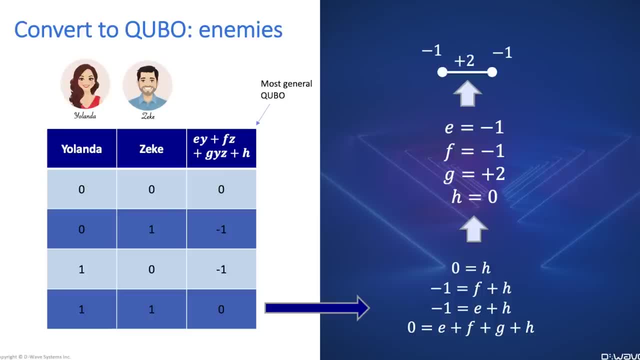 this one is the same as it was previously: the minus one, minus one, two solution. And in this case there's no constant. I don't need to set a constant Or set the constant to zero either way, because the lowest energy in this case is going to be minus one. 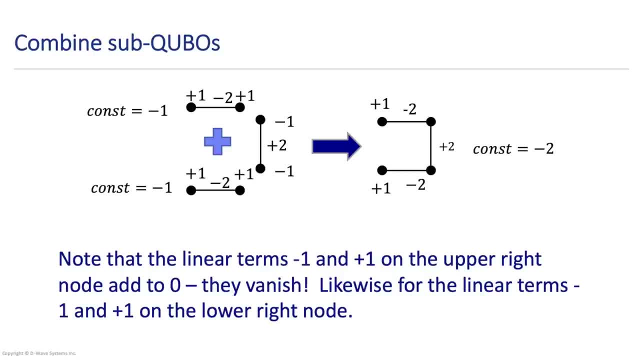 when they're enemies. And then we bring the sub-cubos together by putting them all on the same graph and you can see in the right side, when we add all these things up, that the linear terms actually on the upper right cancel. And likewise for the linear terms. 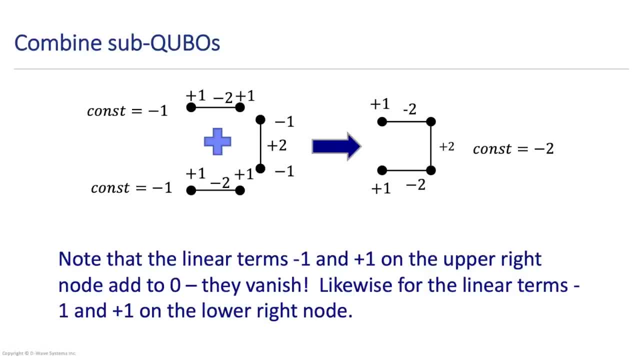 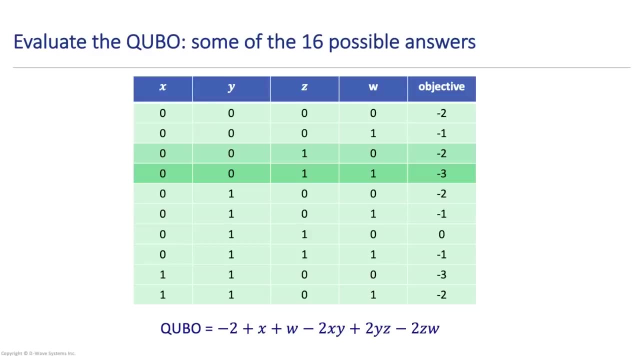 terms on the lower right, and we end up with an overall constant of minus 2, because I put a minus 1 on that 1, 1 minus 2 relationship, and so my result in cubo is shown on the bottom here with, as we see, the terms like minus 2xy and so. 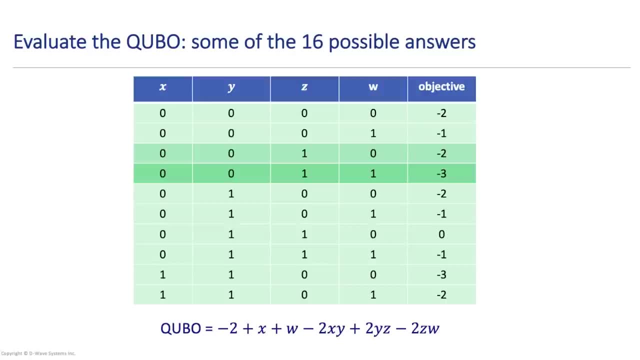 on the cross terms and also some linear terms in X and W, but not Y and Z, and the constant of minus 2, and when we run this, which I'm not showing- we see that we have two solutions that have energy minus 3. you can see that there in the 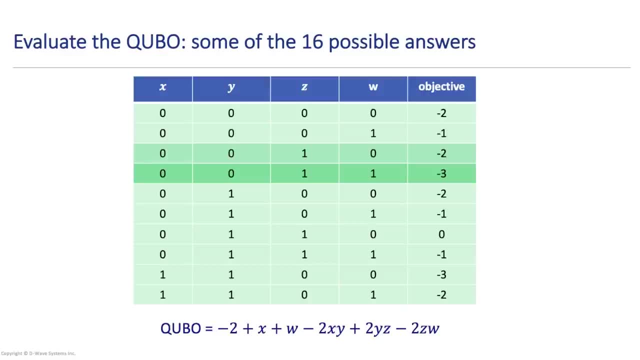 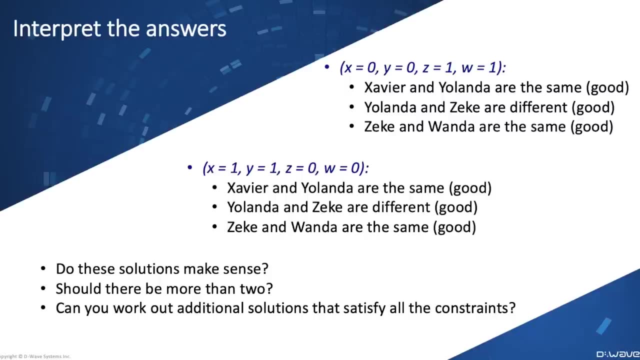 fourth row and then the row second from the bottom. so now we interpret these answers and do they make sense? if we look at the first one, x equals 0, y equals 0, z equals 1 and W equal 1. yes, the x and y relationship are the same. the y and z relationship are: 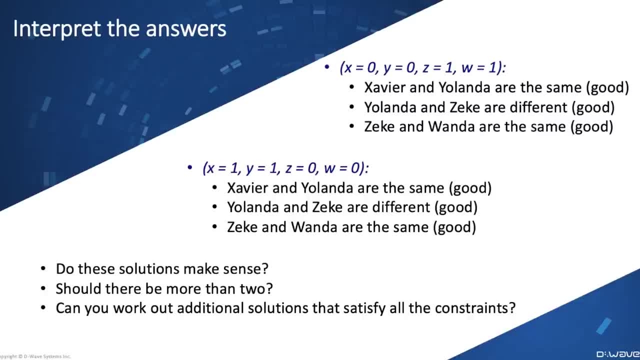 different. that's good. and the z and w are are the same, which is also good, so that solution is valid. and then I can also look at the other one: x equal 1, y equal 1, z equals 0, 0 and W equals 0. is that valid? and the answer is: x and y are the same, that's. 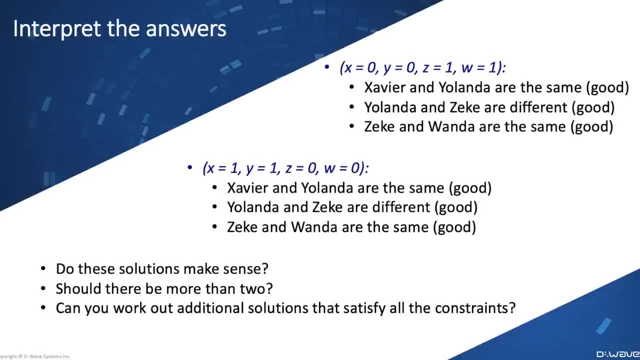 good. y and z are different, that's good, and z and w are are the same, which is also good. so it seems like these. the solutions do make sense. they're valid should there be more than two. can you work out any additional solutions to this that satisfy all the constraints? and I think, if you think about 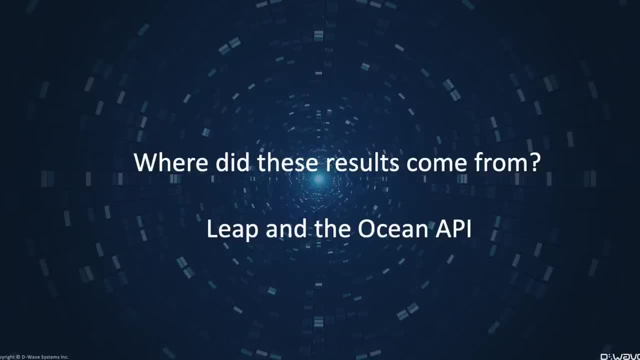 it for a while, you'll find that you can't. it's only two choices for that first qubit, since we're in binary math here, but think about it anyway. it's a fun thing to think about. so the next question is: where did I get these? 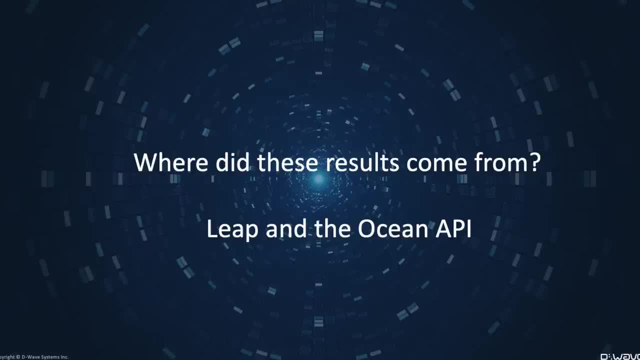 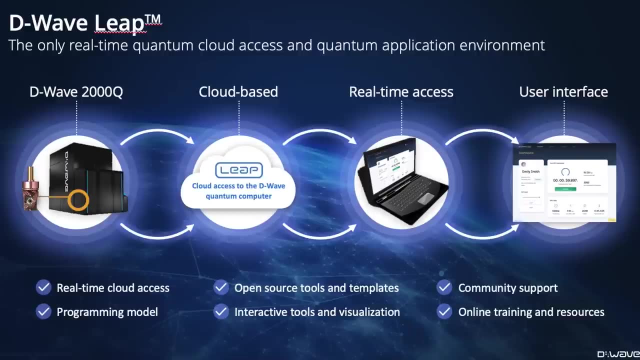 results. where, what, how did I do this? and so that means that I need to introduce you to leap and the ocean API. leap is a cloud-based access platform for the d-wave quantum computers, and so you just access it through the infrastructure. your jobs, basically from you, are sent through the cloud onto the 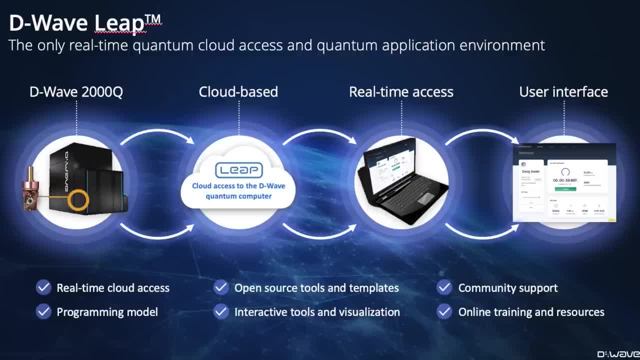 solver and sent back, and you can sign up for free. I'll provide the link at the end. in your first month you get a 1 minute of free qpu, which is actually a lot, and i should say that's actually leap time which you can use on a QPU or on a hybrid solver, which we're not talking about today. 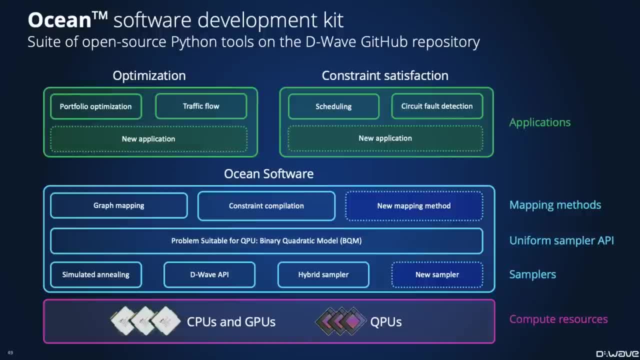 But let's turn next to Ocean, and Ocean is our Python programming API. The lower levels abstract away the details of speaking to the solvers and then you move up, if in a pictorial layer sense, if you remember the OSI interconnect picture for networking. 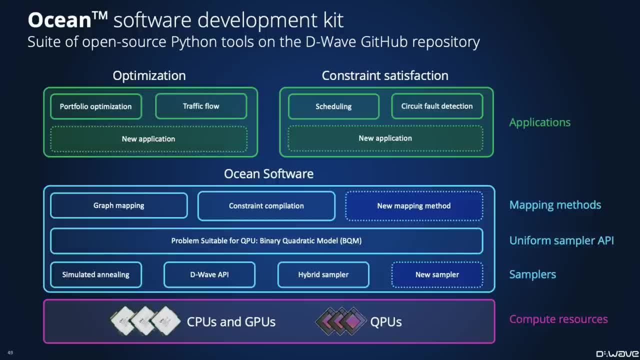 Samplers and solvers at the next level, then, as we saw earlier, the binary quadratic model, model, abstraction between easing model and OSPF, and then up to specific problems all the way at the top, like portfolio information, portfolio optimization and portfolio optimization, Traffic flow and so on, and so programs are written in Ocean and then sent to D-Wave. 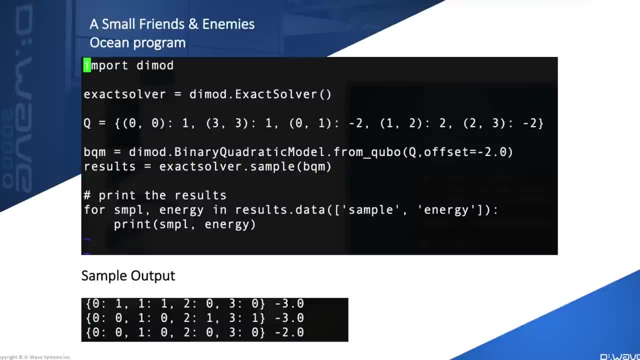 using the LEAP infrastructure And here's a very small problem that we can run using the Ocean infrastructure. This particular Ocean program does not actually use the QPU itself. It uses a small solver called ExactSolver which can work for QBO problems which are so small that you can work through all the options. 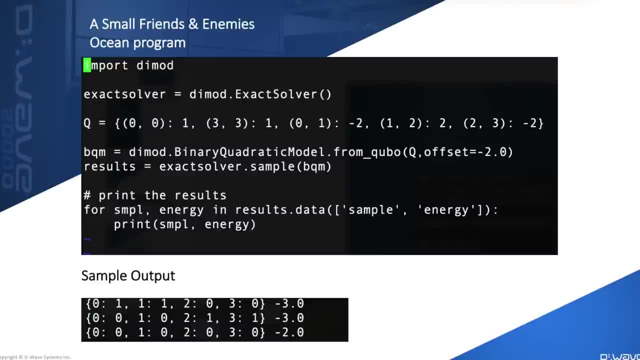 But in the code we have an import. then we define the solver itself, We call it well, we refer to it actually, and define the QBO in that Q matrix and some things there that we'll talk about in a different unit, creating a binary quadratic model. and then we run. 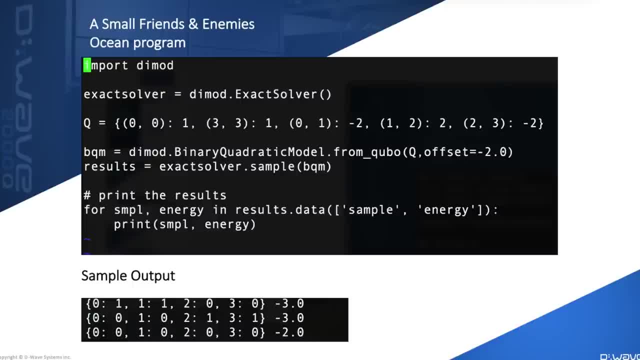 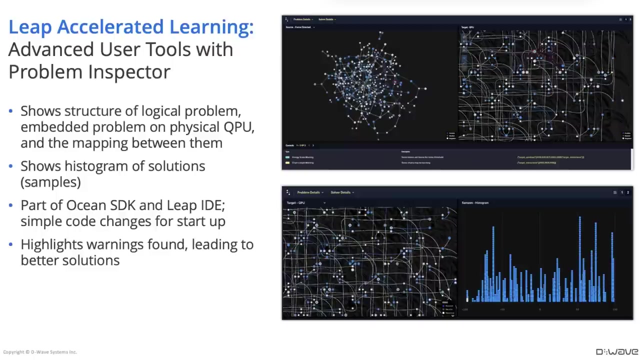 the problem. that's the line ExactSolver dot sample and finally print the results And if you look below, you can see two rows with energy minus three, indicating that the solver has indeed found the right solutions that we discussed before. Now I want to mention some other features of LEAP which have been added to make programming. 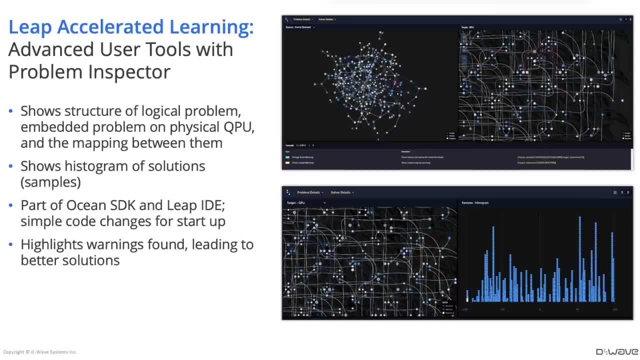 a lot easier on the D-Wave, And one is the problem inspector, and what you see here are some screenshots. The logical problem that you submit is shown along with the problem as it actually lands on the QPU, which involves something called embedding, And please tune in to the second part of this tutorial to find out more about embedding. 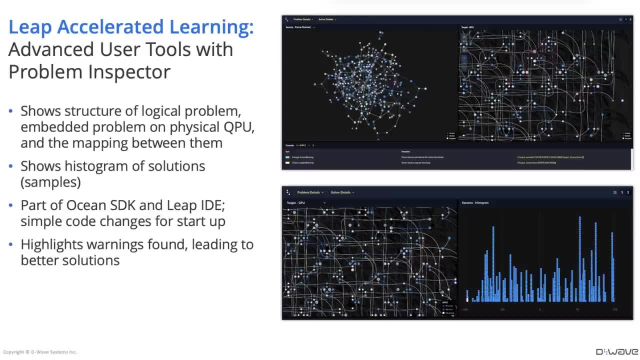 But you also get a histogram of solutions and the warnings that have been found, And so the inspector really is a good way to see how your problem is actually running and details of it that you might want to make use of to do tuning to make it run even better. 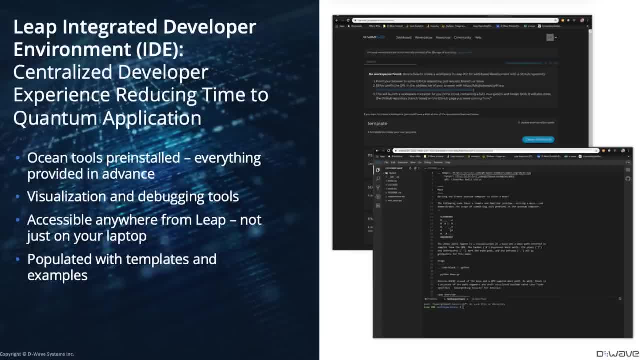 And another feature of LEAP is the LEAP integrated developer environment, where it's basically an IDE, a programming environment for you, where the Ocean Toolboard, which is a tool that you can use in the cloud, can be installed on the D-Wave. 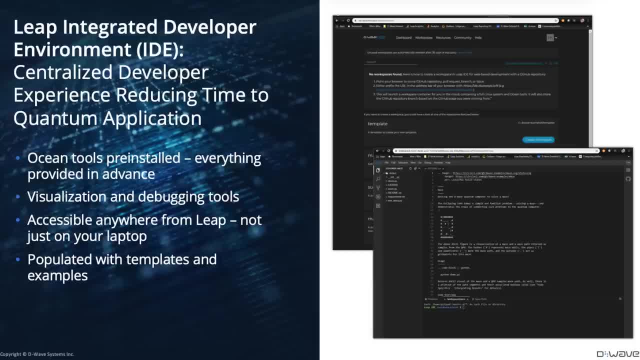 And you can use it in the cloud so you don't have to download anything. But it's also populated with templates and examples from the D-Wave collection of examples if you wanted to contribute to the Ocean Toolkit or even just explore some of the problems which have been solved. 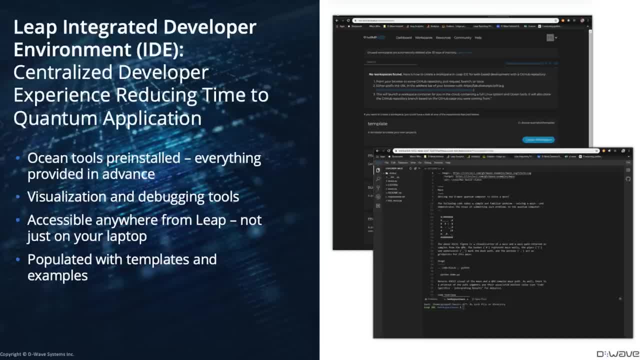 So please also check out the link in the description for the link to the Ocean Toolkit And if you have any questions, please feel free to reach out to me and I'll be happy to answer any of your questions. And I'll be happy to answer any of your questions that you may have in the future as well. 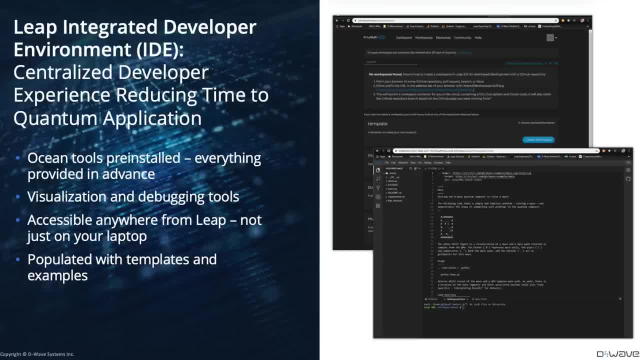 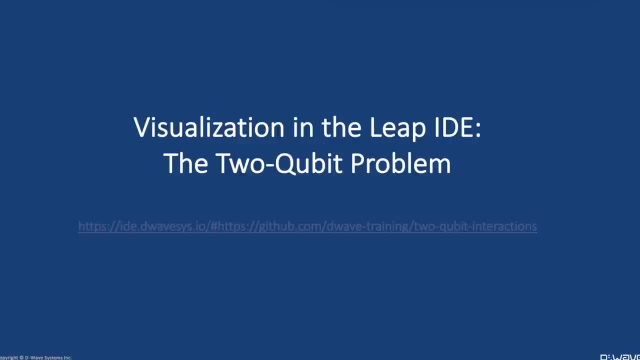 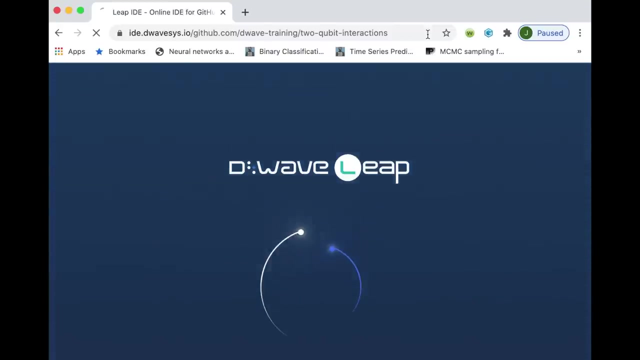 So thank you so much for watching this video and I'll see you in the next one. Thank you for watching this video and I'll see you in the next one. Thank you for watching this video and I'll see you in the next one. 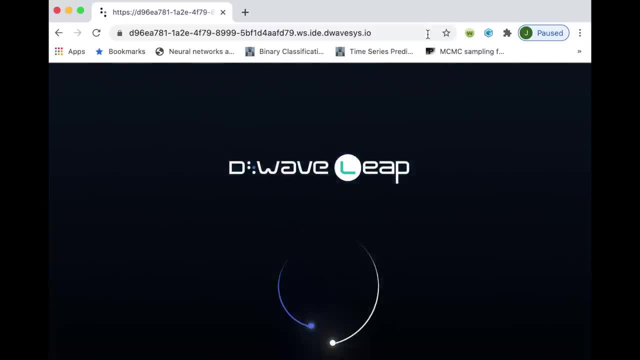 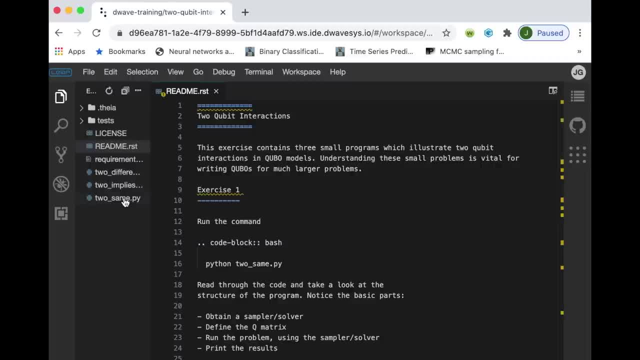 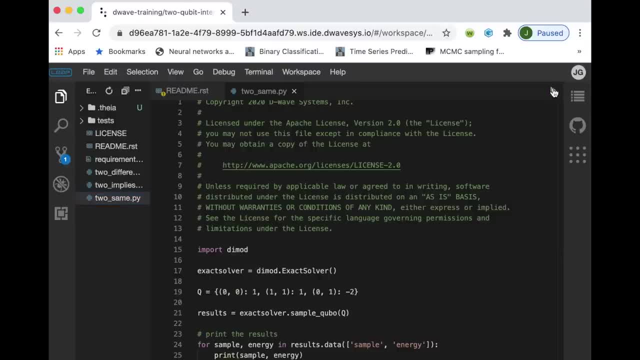 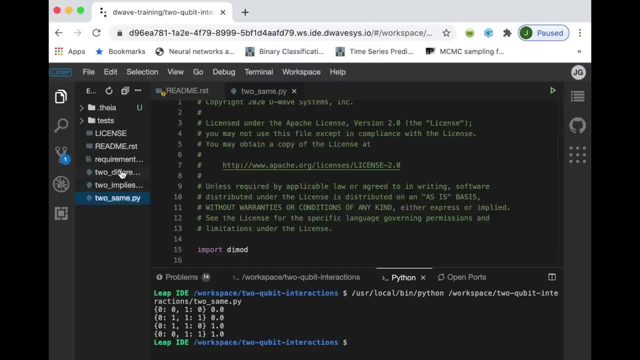 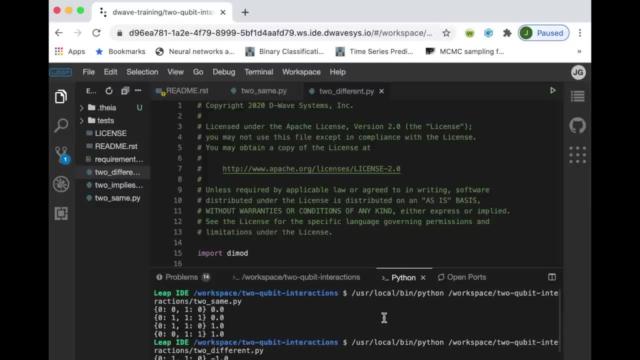 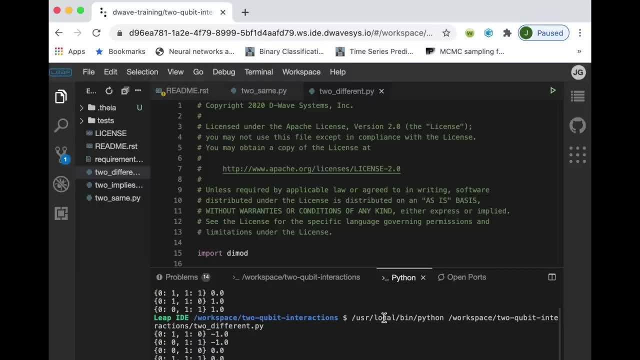 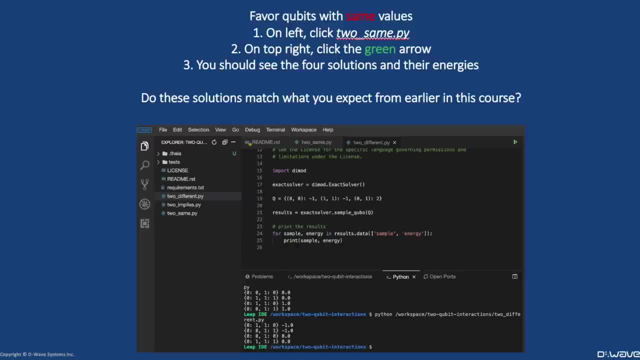 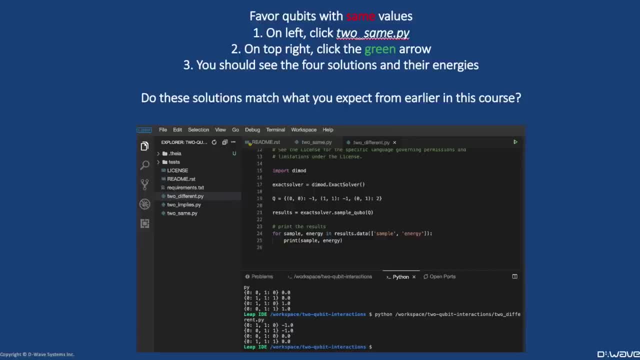 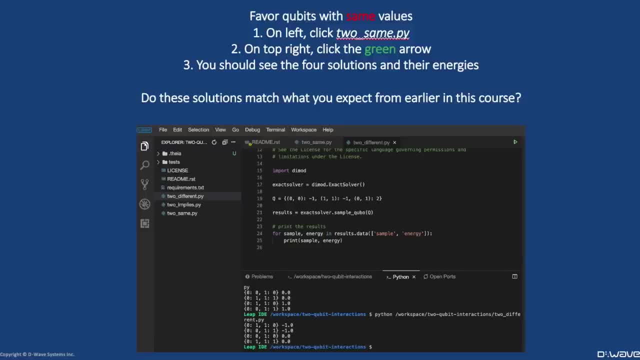 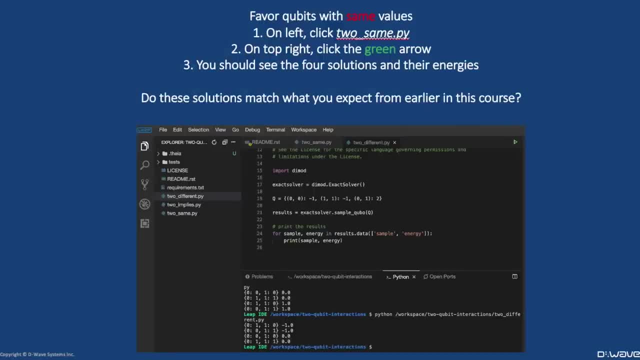 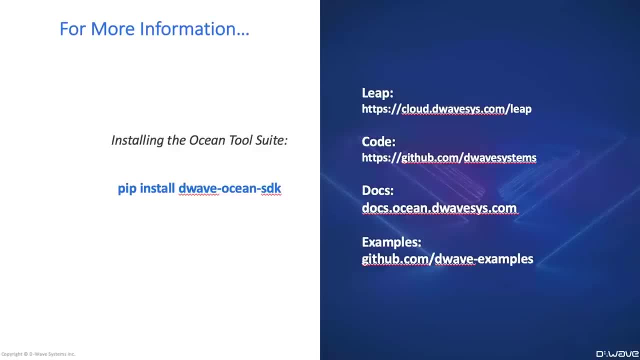 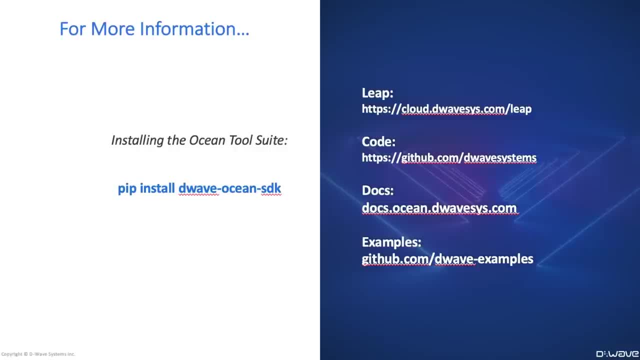 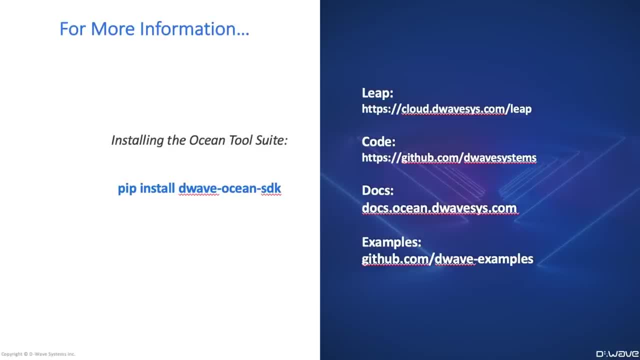 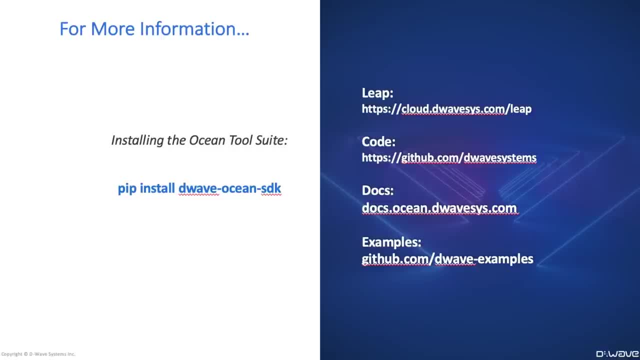 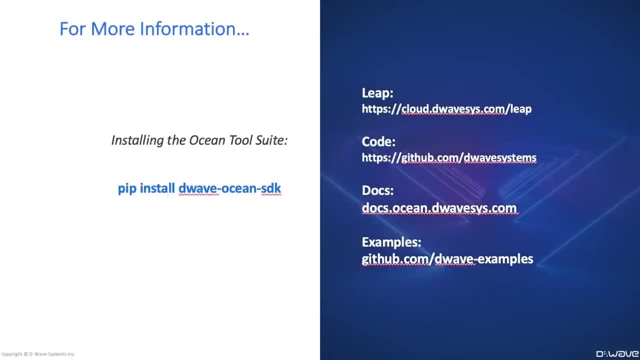 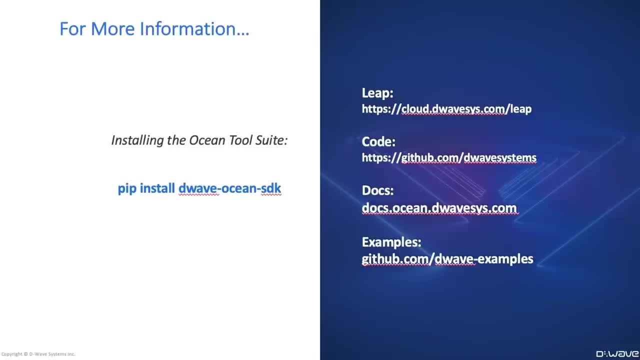 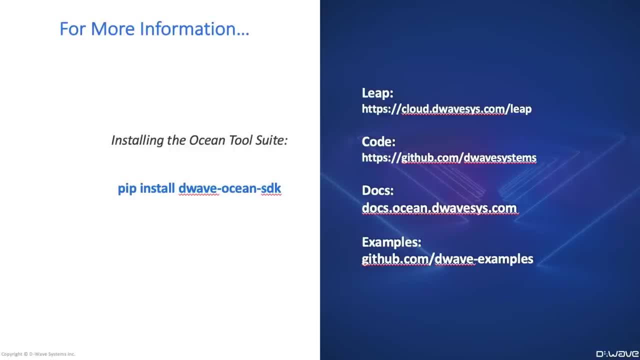 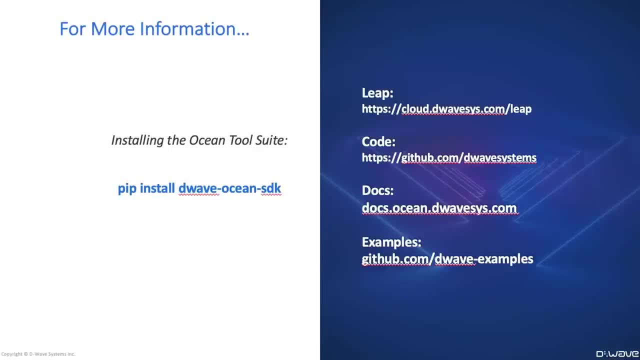 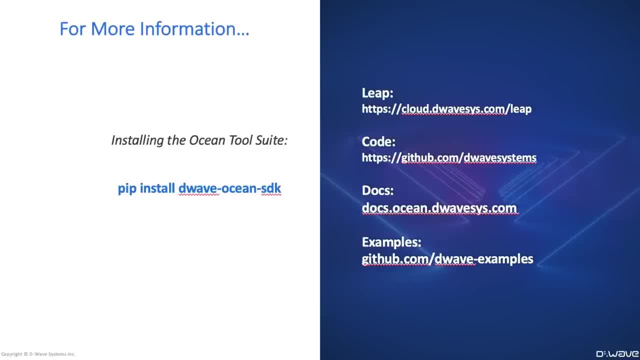 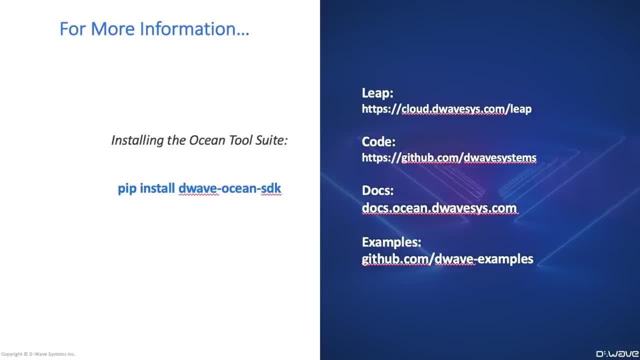 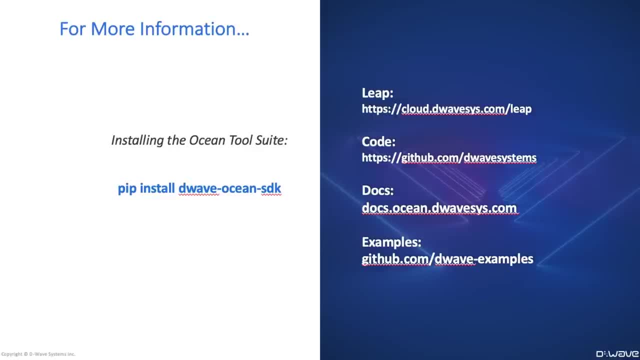 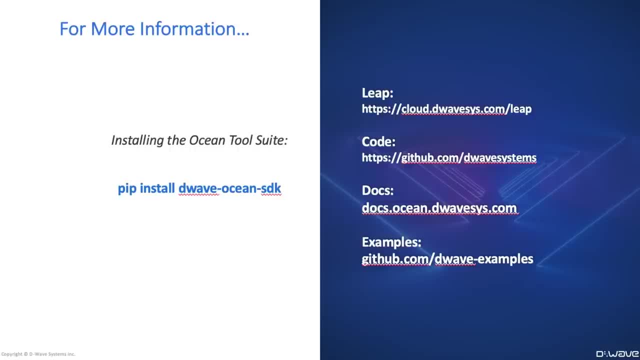 It's a good starting point. And also on the left is how to install the D-Wave Ocean SDK from PyPy with just the pip command, and I encourage you to do that so you can get started. I often tell people: get started on this programming as soon as you can. 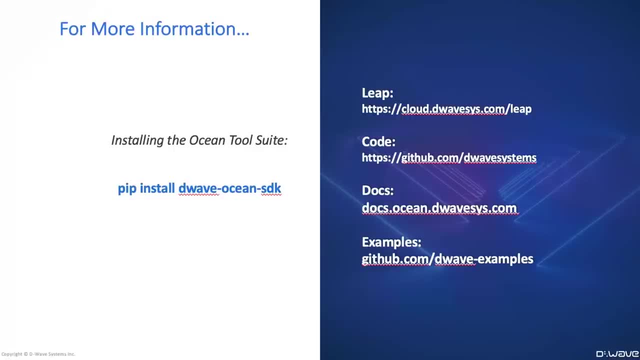 because it's changing. This is what's happening now. We're at an early stage in this field, and the more you learn about it, the sooner the better, So you can then deal with the changes and the new information as it comes. 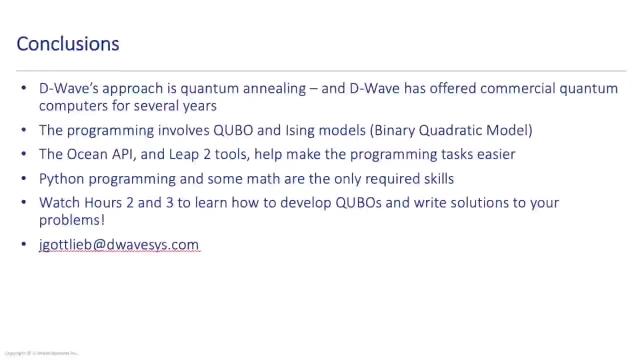 It's the only way I think we can really keep up. Okay, so it's time to wrap up this first hour of the three-part Practical Quantum Computing. This is a tutorial by D-Wave, And so some conclusions are that D-Wave's approach is quantum annealing. 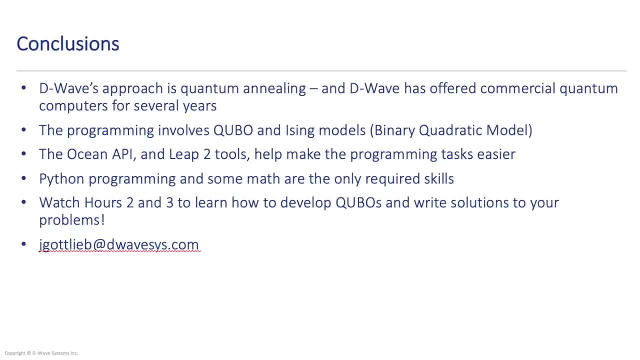 You now know a bit more about it, and you know that we've been offering commercial quantum computers since 2007.. The programming involves cubo and easing models, which can be summarized as binary quadratic model, So that's something that you need to be familiar with. 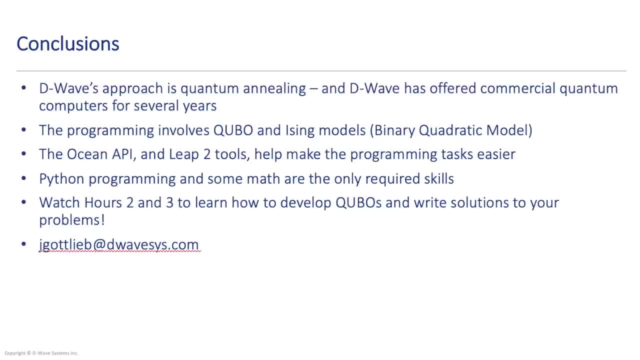 and we went over Some very simple but very important problems, just even two qubits, And it's sort of interesting for me that people often send questions about very complicated things and I'll refer back to the two-qubit problem and say: are you familiar with it? 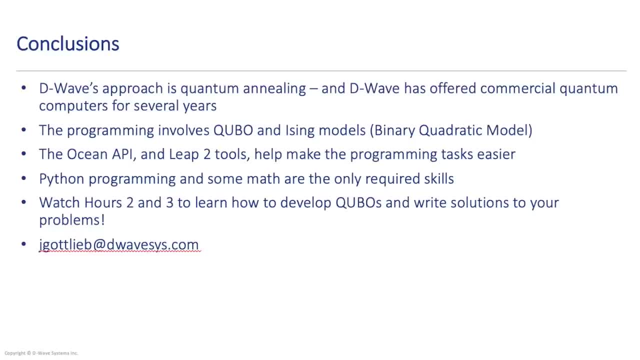 And I think it feels to them like they're getting sent back to high school or something. but that's not what I want to do. If we start on the same page and we understand the basic problem, then we're in much better shape to understand the answer. 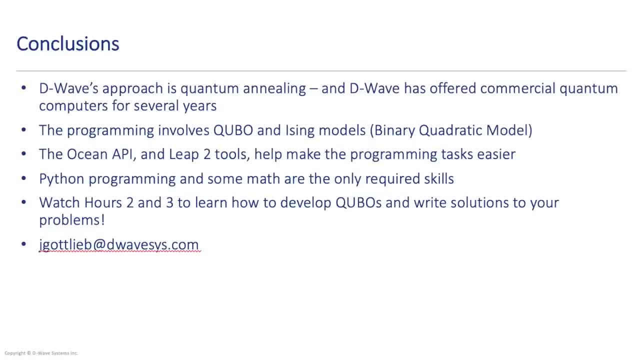 So that's one of the things that we're going to focus on in the next few weeks. The D-Wave Ocean API and the Leap tools make the programming easier, And you really have to have some skill at Python programming And I believe the mathematics is algebra, nothing beyond that. 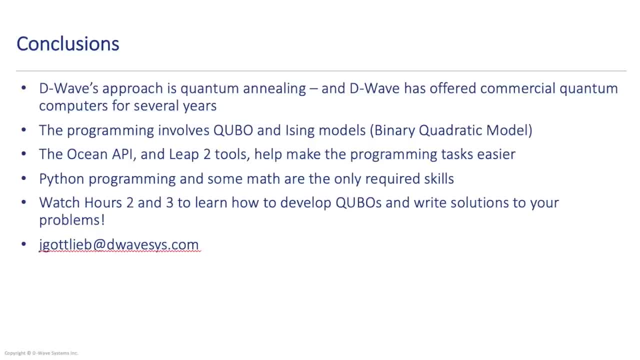 And, as I said, do sign up for Leap, Get that one hour, excuse me, get that one minute of time for Leap. And then I should mention, before we close, that if you provide a GitHub ID for open source development, that you can get one minute free once a month.